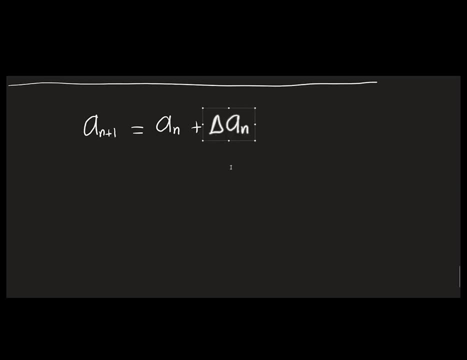 change happens during the interval of time. Okay, one more example I'm going to do with that is this one here. So this is an example about the mortgage of a home. Okay, so let me read. So six years ago, your parents purchased a home by financing $160,000. 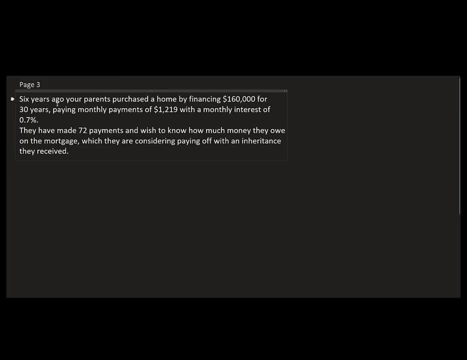 for 30 years, paying monthly payments of $1,219 with a monthly interest of 0.7%. So that's very standard. The interest is monthly, something like that. Actually it's kind of cheap. They have made 72 payments and wish to know how much money they owe on the mortgage. 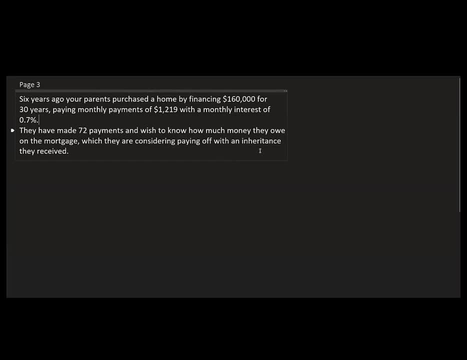 which they're considering paying off with that inheritance they receive. So what we need to do here is, with all this information that is up here, they already made 72 payments, So we want to know how much money they still owe on the house. 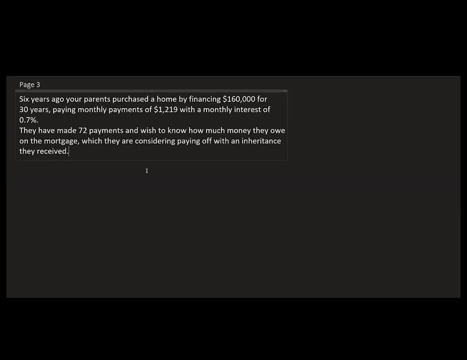 Okay, so let me, Before we start doing anything about that, let me ask you some questions about the mortgage of a home, Of a home. Now, when you hear this, what comes to your mind? What should go here? the mortgage of a home. 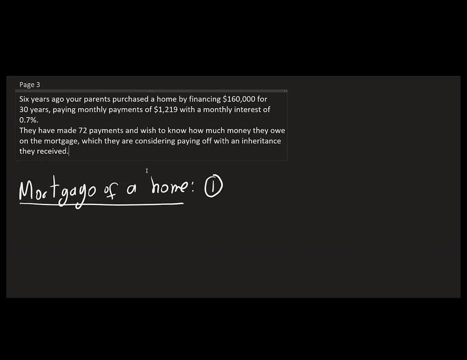 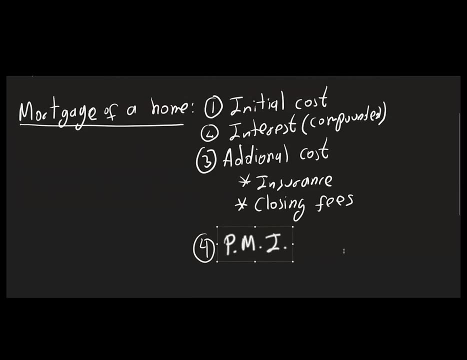 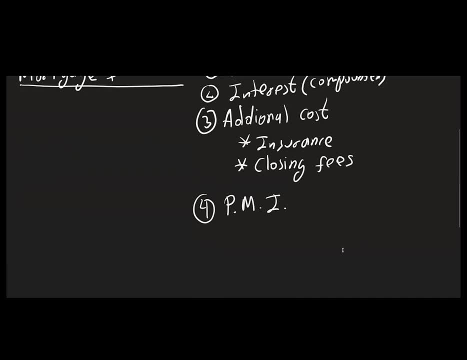 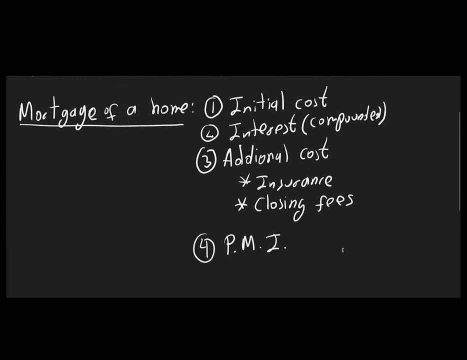 extra interest. So, for example, if you have a house that cost, let's say, two hundred thousand dollars and you pay five percent down payment, then you have to pay an extra interest on that. So some of the people who you're borrowing money from they might not tell you this, but they're gonna add this if you don't. 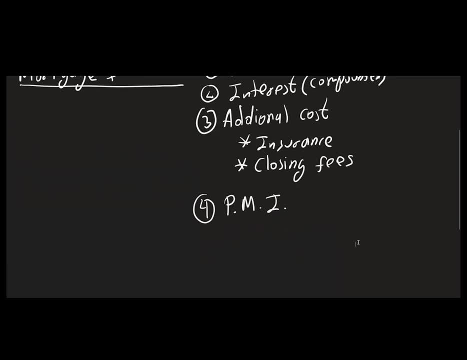 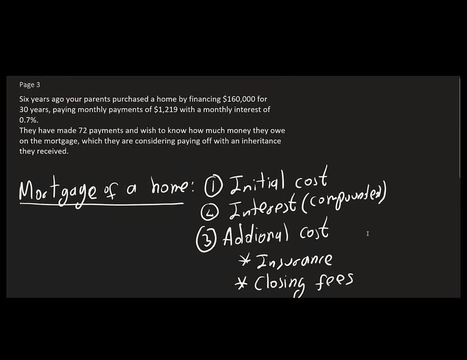 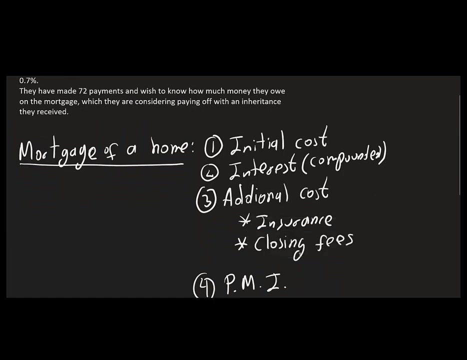 have that, that 20% down on your house. Okay, Alright. so how we're gonna solve this problem here. We're gonna simplify this and we're gonna- and we're not going- to take into consideration the closing fees insurance the PMI. 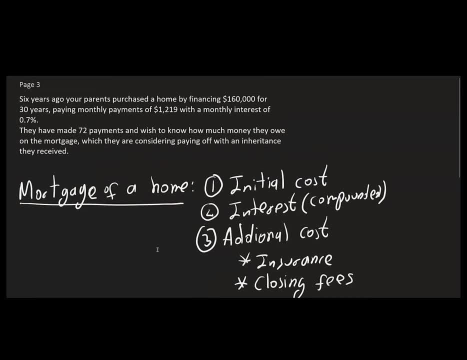 if there is any or any initial cost or anything that you have to do with the house, like you have to maybe get it, you have to check if the house is doing well. all all of that, all those checking that you have to do at the beginning. so we're 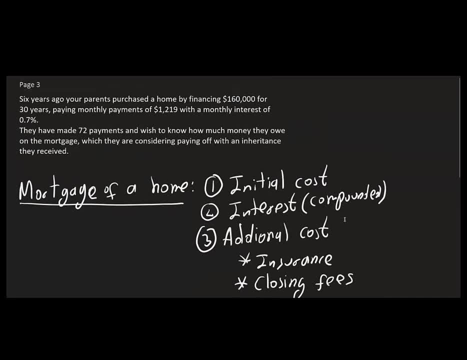 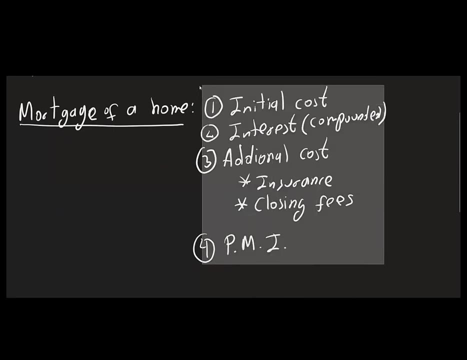 just gonna simply do this. why? because we are simplifying the problem. remember, at the beginning of the class we mentioned that when we look at a problem, but first we're gonna approach it, making some assumptions to make things easier. now, if you take all of this into consideration, then then the problem is gonna be more. 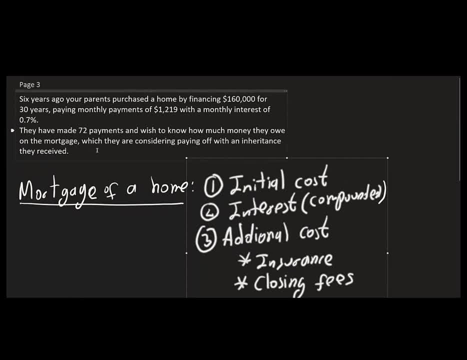 complicated and we probably need to have more information, more than this, but at this point we're gonna solve the problem just the way is stated here. so we're just gonna look at the monthly payment and the interest and that's all. so that's how we're gonna go about that problem. all right, so before we go into 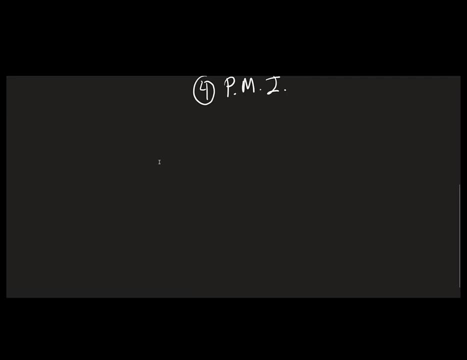 the, the how to solve the problem. so let me draw a picture here using our sequence, the sequence that we always use. so let me draw the picture. so we start here at a zero, which is gonna be our initial value. but before that, before that, let's write. 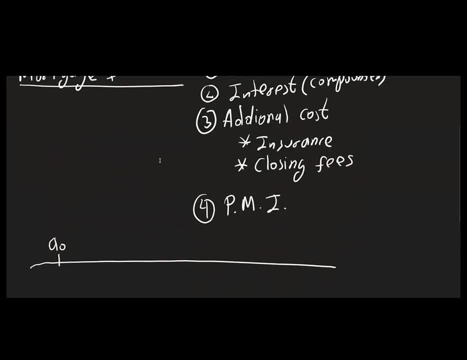 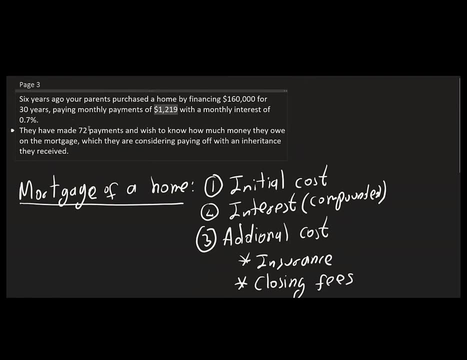 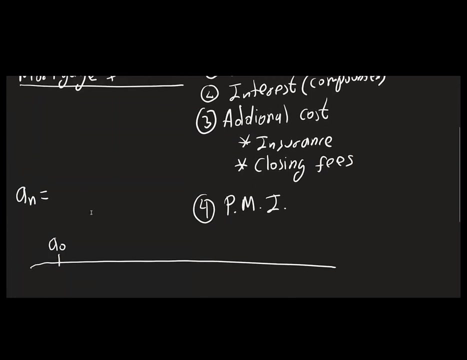 down what a? n should be. now the problem is talking about. let me go back here. the problem is talking about how much we own, so it would be nice if we call this a? n: the amount of money that we owe, or the your parents. oh, at the end of the nth. 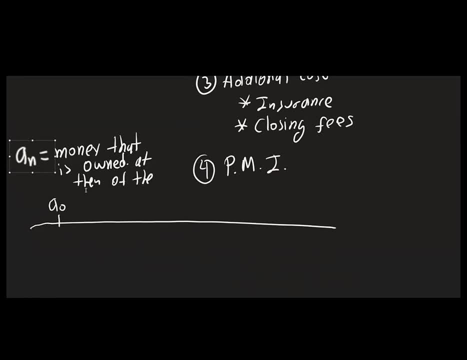 month of the nth month, right. so I'm gonna erase this here, because this is apart of the common value of this video. so this variance- De Brothers said it was about 100 percent, but for my own часов. So let's do this, do the picture here of what we have. 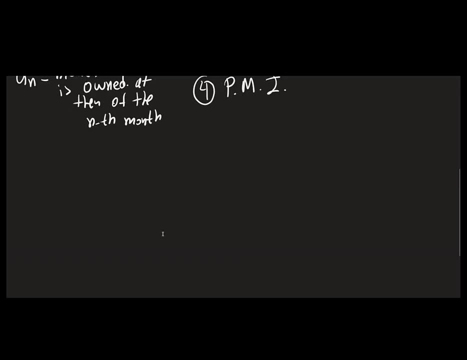 So that would be for us A in. So let's look at the picture, So let's look at the timeline. So this is gonna be A zero, A one. So for us A zero because in this case, the amount of money that we are borrowing 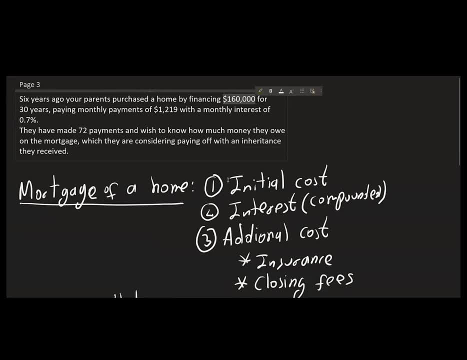 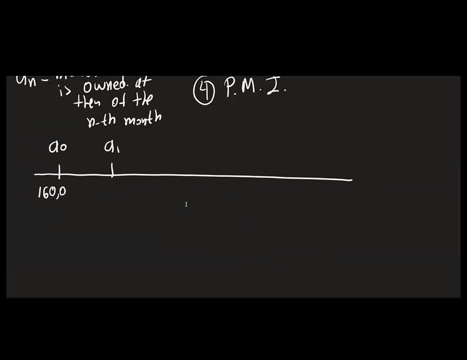 is this $160,000.. That would be the A zero for us. So this will be $160,000. And A one here will be what we owe at the end of the first month. So this period of time that is between A zero and A one. 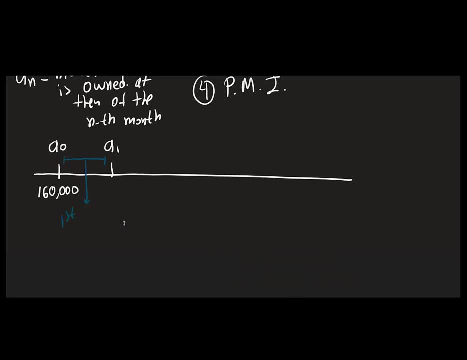 is: this is the first month, And so on. So we have A two and in general, we're gonna have here A in And A in plus one. Now, if we are looking in general at a month, what month is this one? 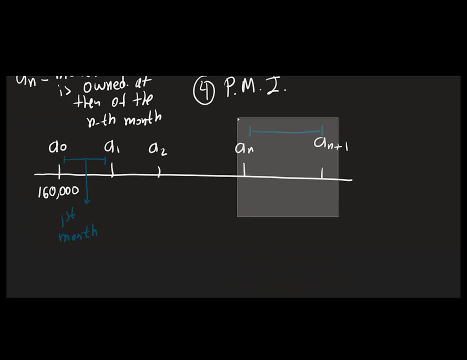 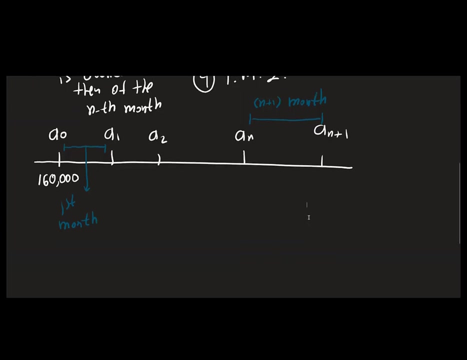 Is this the nth month Or is this the n plus one month? This is the n plus one month, So that will be the n plus one month there. Okay, so let's set up again our try to set up our difference equation here. 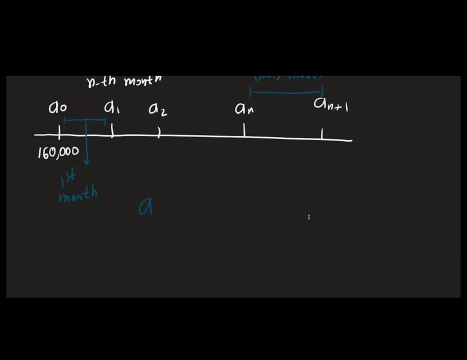 So, as always, we want A in plus. one equals to A in plus the delta of A in, And the idea most of the time is we want to look at what this delta of A in is in terms of the value of A in And remember this: here is gonna be the change that happens. 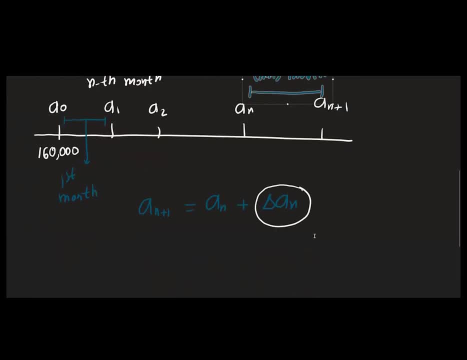 This is the change that happens in this, And plus one month that is here. So let's look at the formula for that. So let's look at that formula. So that will be the delta of A in. Now this is gonna be similar to the problem we did last time. 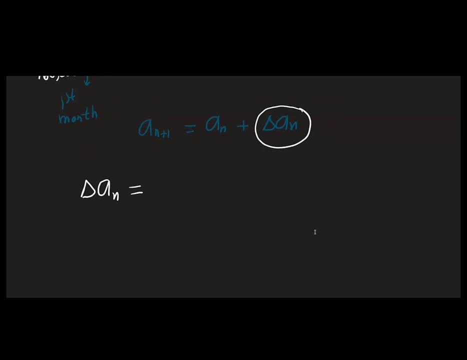 about the saving certificates, when you have some interest and you take money out? Okay, so let me ask you this question: What is the change that happens in this month And the n plus one month, Exactly, interest is added and the payment is made. 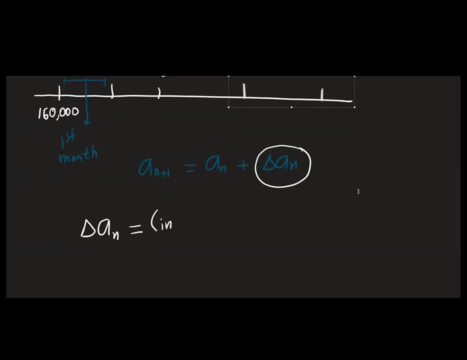 So we're gonna have some interest And then the payment that we make here Now. for this payment, should I put here in the middle? should I put additional or subtraction? All right, so this is gonna be the interest that we are paying. 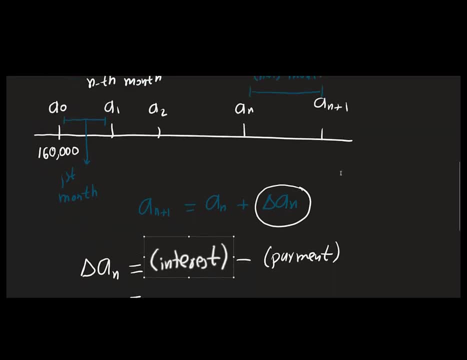 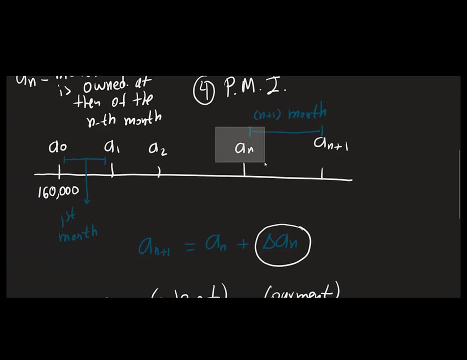 And the interest that we are paying is the interest that corresponds to this month. So that would be the interest over the amount of money that we owe so far, which will be this A in. that is right here. So that will be whatever amount of interest we are doing here. 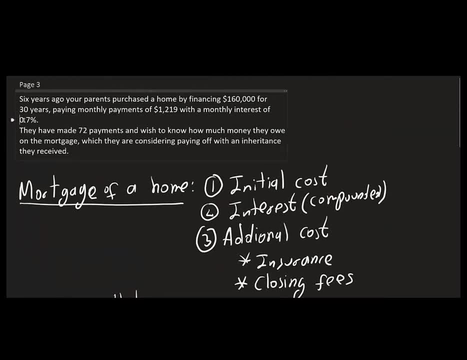 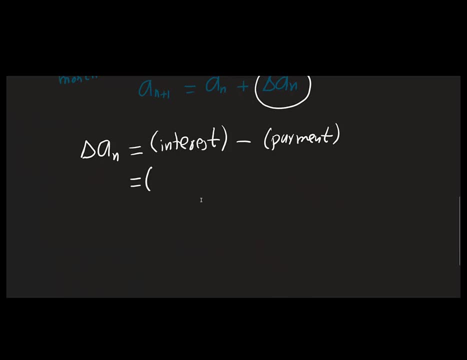 which in this case, according to the problem, is 0.7%. So this is gonna be: the interest is gonna be 0.7% of the value of A, in which is the starting what we owe at the beginning of that month, minus the payment. 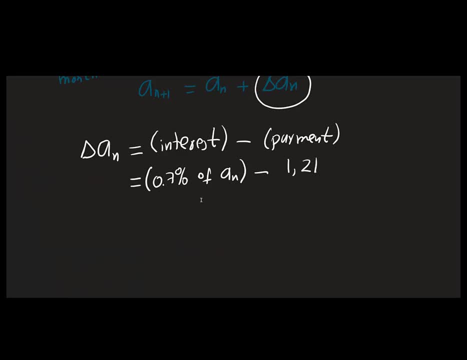 which is 1,219, and that's the payment we are making. okay, So, as we did with the previous example, so we just take the 0.7% of this A in, and that is the same as multiplying by 0.007 of A in. 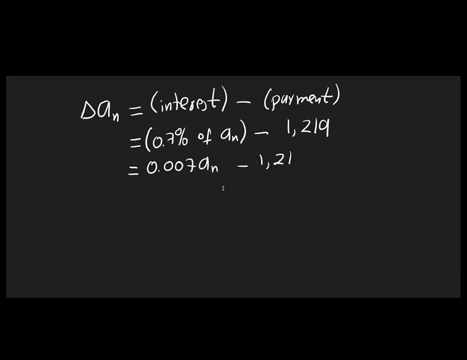 and then the minus 1,219.. So that's gonna give us the expression for delta of A in in terms of A in. So then let's go back again to our original, our way of to set up things. So A in plus one is equal to A in plus the change. 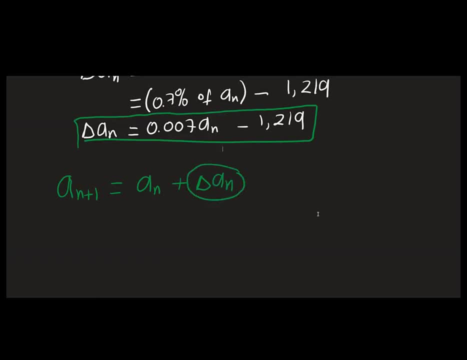 which is delta of A in, and we already know that this change is just right here, which is that formula. So we just have to replace it there to be able to find the recurrence formula. So it's A in plus one equals to A in plus 0.007 A in. 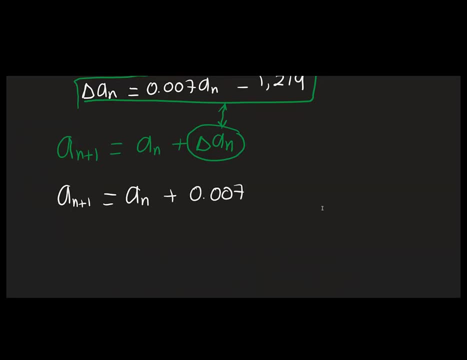 minus the 1,219 that we have there And we just have to simplify now. Look at the common terms here. So I have a one times the A in, So this is gonna give us A in plus one equals to 1.007 of A in minus 1,219.. 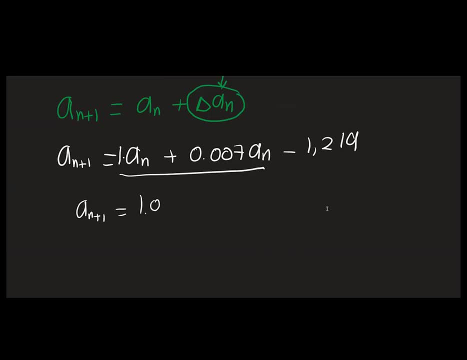 So this is gonna give us A in plus one equals to 1.007 of A in minus 1,219.. Okay, Okay, 1,219.. And this will be our recurrence formula here. So to complete the difference equation, let's look at the initial value here. 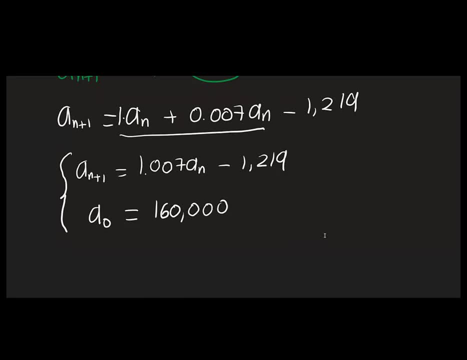 So 160,000. So that will be so. this will be here our difference equation for what we have so far. Now we are almost actually done with the problem. It's time for us to go back to the actual family stock. What we wanna do is we wanna do the same thing. 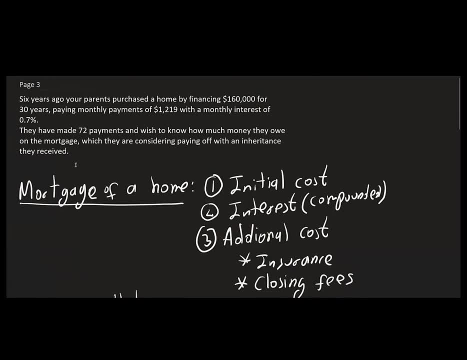 in the initial value. So what we wanna do is we wanna look at the actual value of the new family stock. So basically, we wanna do the same thing we did in the initial value of this family stock. Now we will have this formula that we created. 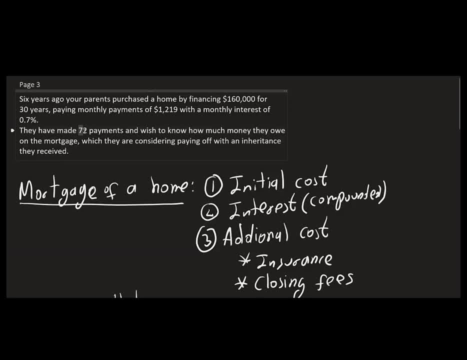 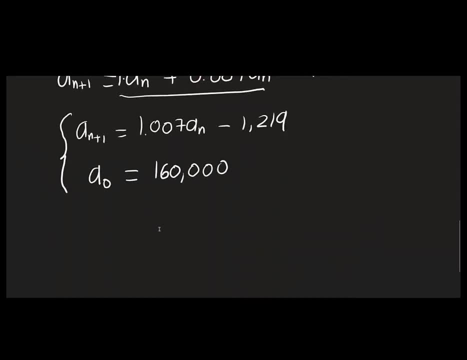 that we have here. Okay, Now we will have, we will have, we will have the value of this family stock. And this is gonna tell us the value of the family stock, Because let's go back again what the statement says by hand, but it's going to take a very long time. Now let me do a couple of them so you know how to. 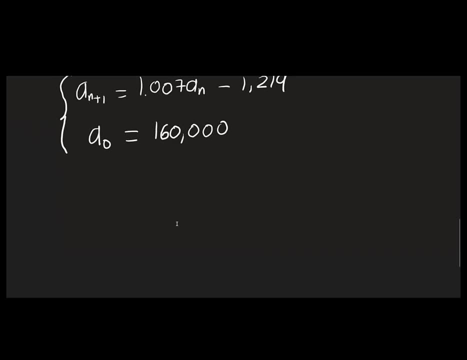 do this by hand, without using Mathematica. So let's say you want to compute the value of what you owe in the second month, which is this one. So for that, what you're going to do is you're going to use the recurrence formula. that is right here, So that's the one you're going to use. 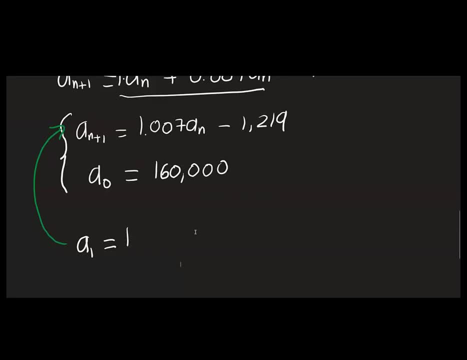 So a1 will give you 1.007. of what a a0 minus 1219.. Now this a0 that is here, this part, is 160,000.. So if we just plug it here, we will be able to know what is the value. 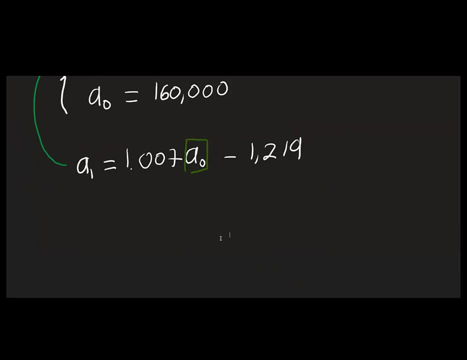 of a1.. Now, if you do all that computation, let's say using your calculator, you're going to get 159,901.. So that will be what you owe at the end of the second month, at the beginning of the second month. Okay, and so how would you do a2? then Let's go a little bit further. just one more before we. 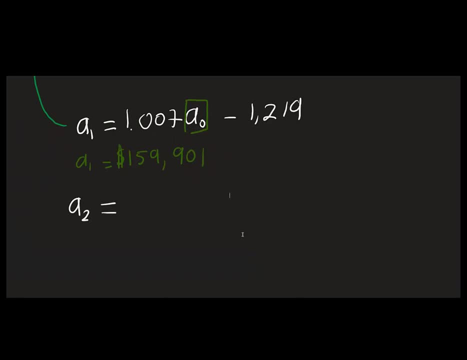 look at Mathematica. So what would be a2? If you were to compute this manually, can somebody tell me what this is going to be in terms of the formula? And now this is again. so the a1 is here. We already know that one from the one before. 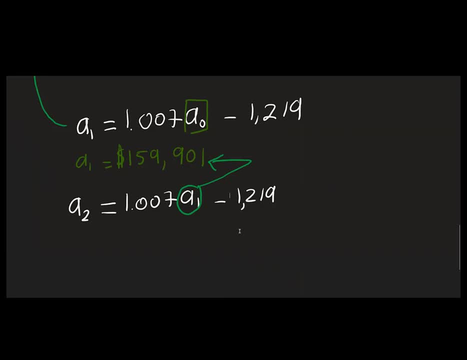 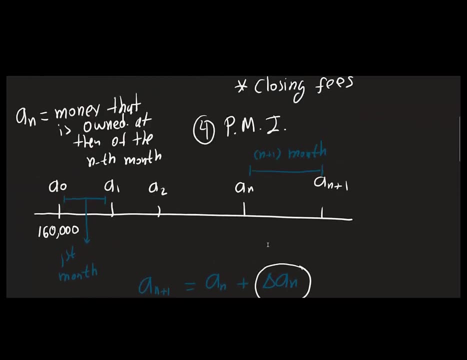 So it's a recurrence formula because it's calling itself many times right, Okay. so of course, we're not going to do this by hand, because it's going to be up to this: How much was it here? The 72 payment? So we're going to use Mathematica for that. 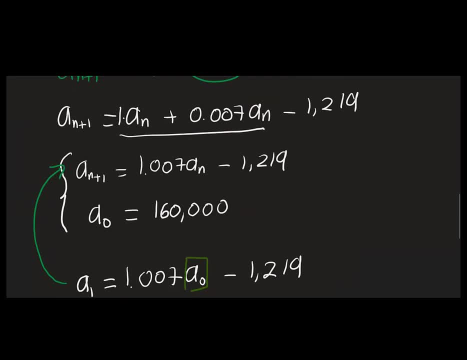 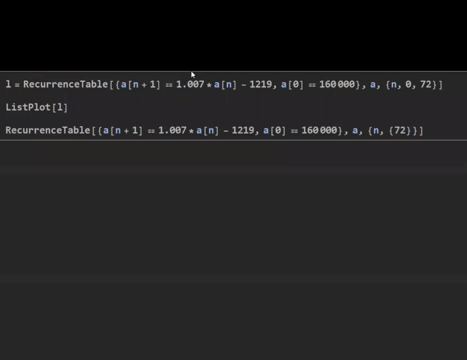 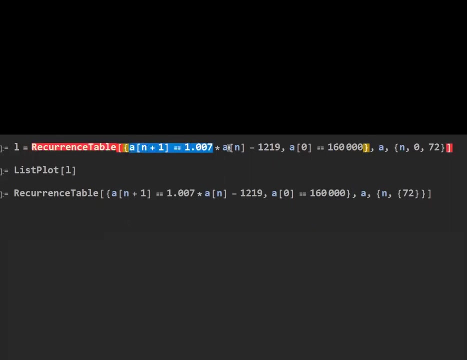 So what I'm going to do now is I'm going to show you the Mathematica code that I have here. Okay, so the same thing. we did the last class. So it's again the recurrence formula, the recurrence table that we have here Inside. here I have the recurrence formula. 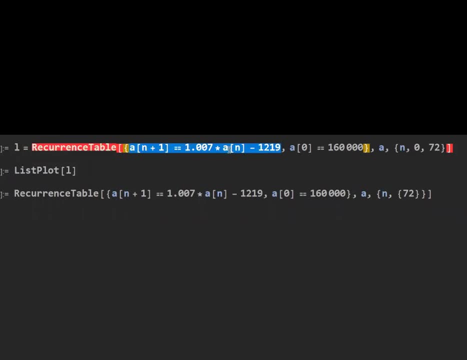 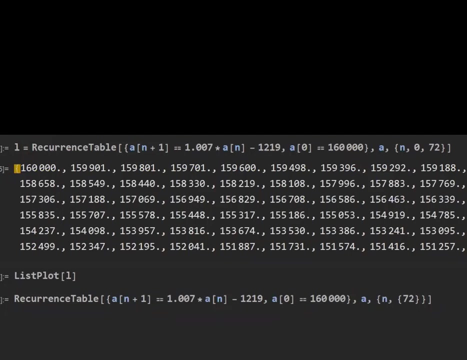 which is a1 plus 1, equals to 1.007, a1 minus 1219.. The initial value is 160.. Our sequence is a. Let's say we're going to go from zero to 72. And so the last value is the one that we're looking for. 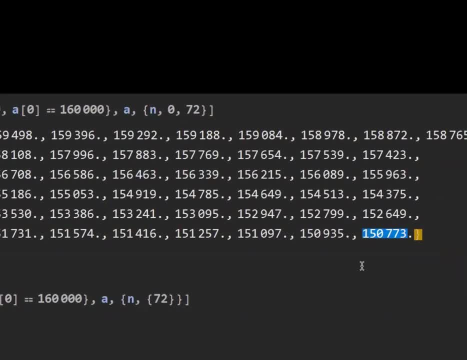 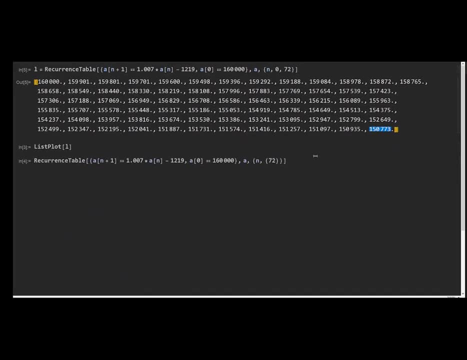 there's one here: 100.. 150,773.. Okay, Now there's another way you can do this in Mathematica. Like you see, in this particular problem I'm only interested in the last value. I don't actually need to see all of this data. that is here. Now we can do that inur. 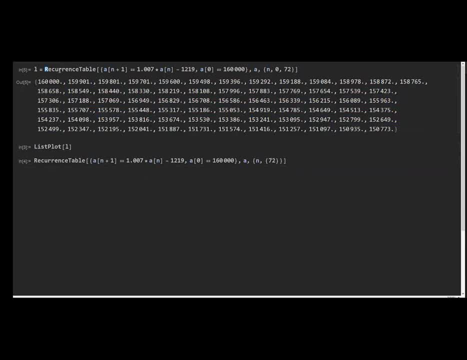 Now we can do that in Mathematica by using exactly the same code, but there is only one difference here. So instead of saying from 0 to 72,, we're going to say just between curly braces, just 72. And if we press enter there, we're going to get just the value that you're looking for. 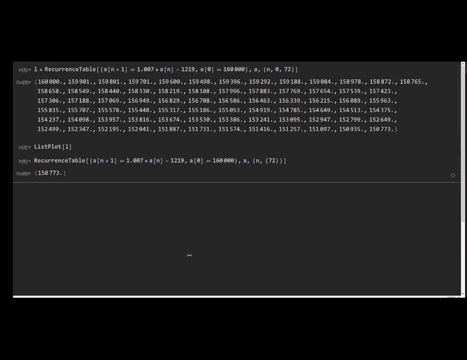 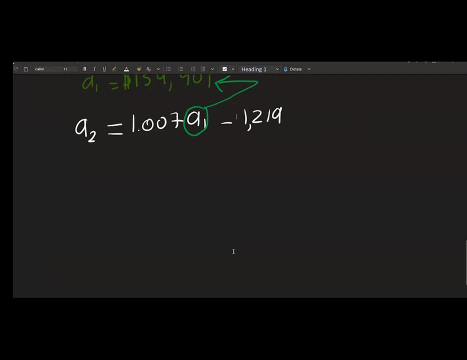 So let's try to. so let's put this in the as an answer. So let's put this as an answer here. So after- let me change into this one- So after 72 payments, which is about six years, Your parents how much did they owe? 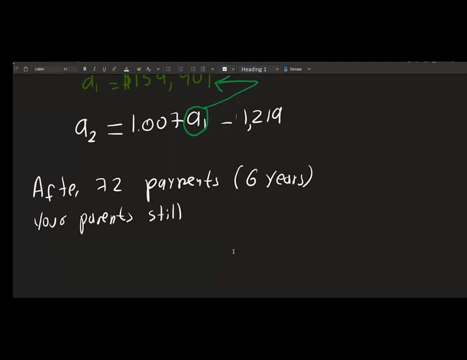 They, the parents, still owe. what was the the number? can somebody tell me? 150,773.. 150,773.. Okay, So I just want to point out this beyond what the problem says is. so look at this. 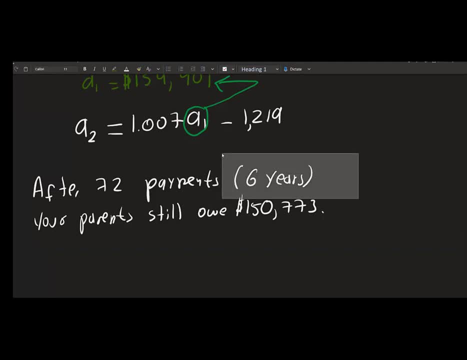 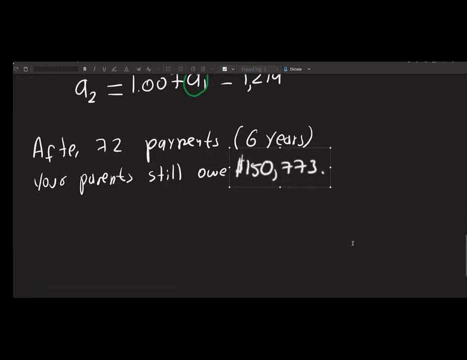 After six years, how much they actually have paid over those six years of the house. The house initially is 100, so the loan that they took was initially $160,000.. Okay, Okay, They only pay a little bit less than 10,000. 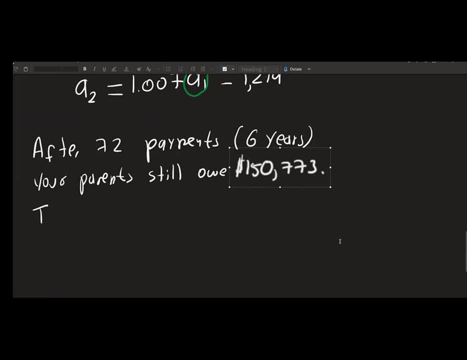 So they have only pay. okay, if you make, the difference would be $9,227 out of the 100, out of the 160,000.. Okay, Okay, Okay, Okay, Okay, Okay, Okay. So this is the total of the 60,000 dollars that they owe. 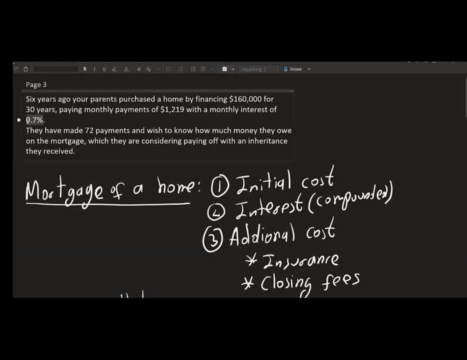 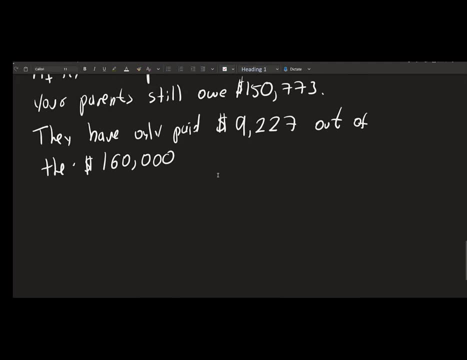 I mean, I'm not exaggerating here. This 0.7% is not a that a high interest. So this just to show you how much money the bank is taking from you or whoever is lending you the money you're. they are ready. Pay. as you mentioned, they already paid uh to the bank, or, or whoever, or whoever lends it to you, and then the money, that was 72 payments multiplied by 1219, which you made it correctly. That's like 87,, like almost $90,000. 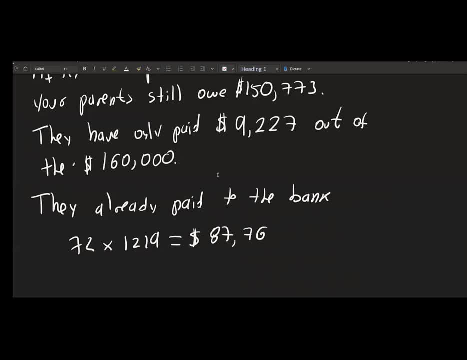 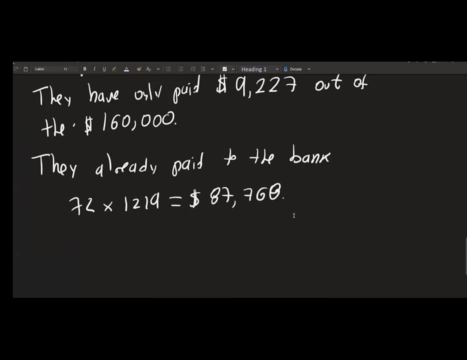 So 87,768.. So it's a good business to lend money, basically, All right. so this part, so this is the section 1.1.. So I just finished the section 1.1 with this example. I'm gonna move into section 1.3.. 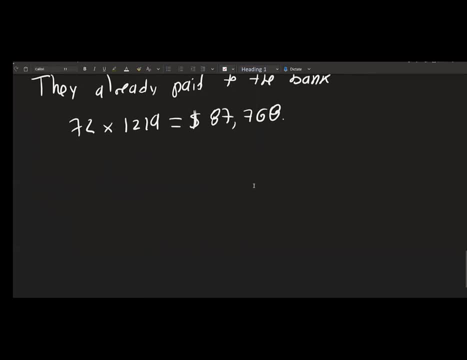 So the section 1.3 is Solutions to Dynamical Systems. So this is the section 1.3. The Dynamical Systems. So I'm gonna say this again. So the reason I'm skipping 1.2 is because 1.2 is the same idea. 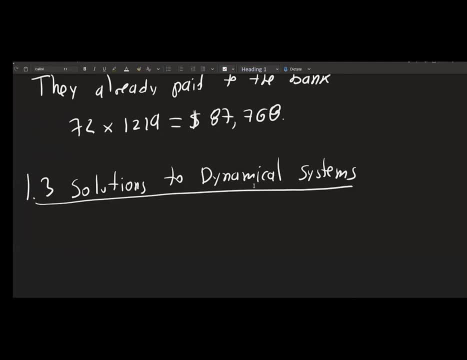 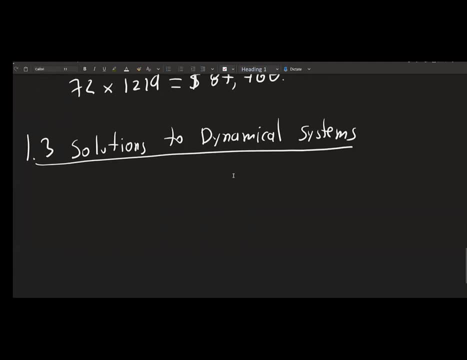 is the same kind of formula we are using. So we are using a difference equation, but it's approximation. So I'm gonna do this one first, because this is a way to solve things exactly. So I'm gonna first give you the solutions of things exactly. 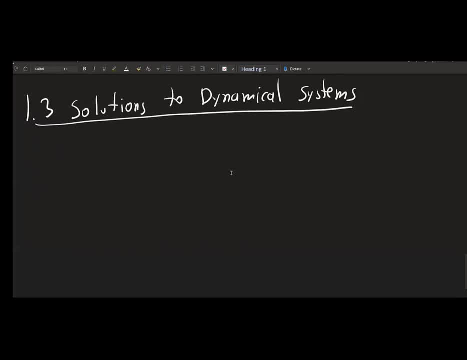 and then we'll go to to examples where we have to do some approximations. So what is the solution to a dynamical system or a difference equation? So what we want to do is is we want to find a formula, find a close. 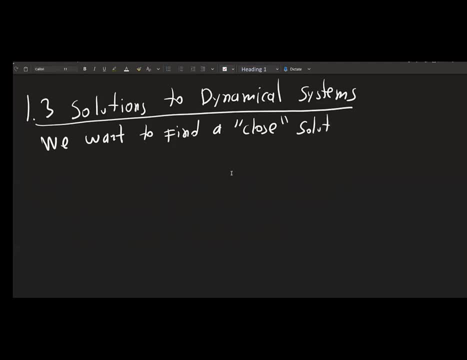 a close solution to a dynamical system. And what do I mean by close? So what that means is that we don't want to use recurrence formulas, So we don't want recurrence, recurrence formulas. The reason we don't want recurrence formulas is because 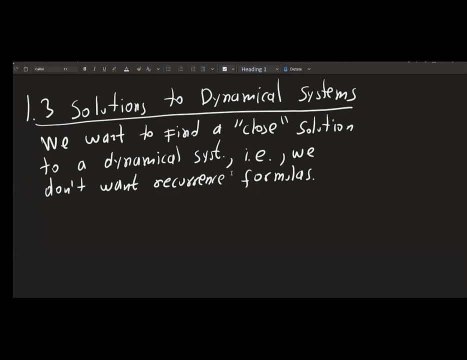 unless, of course, you use a mathematical hypothesis, that you always have to rely on the previous computations to get to the next one. So when you have a recurrence formula, the disadvantage is that you need to rely on the previous computations to get to the next one. 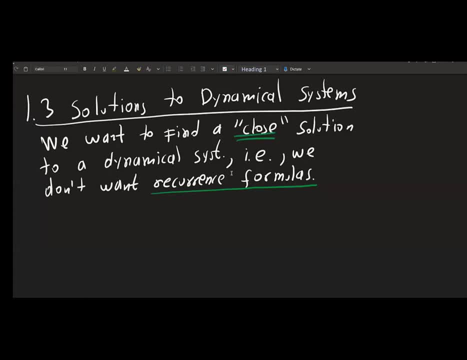 When you have a close formula, you don't have to do that, You don't need, you don't need to know the previous computations And to do that we're gonna use this theorem here That is gonna tell us. I'm gonna call this theorem number one. 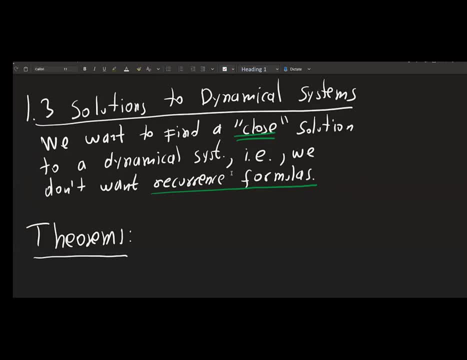 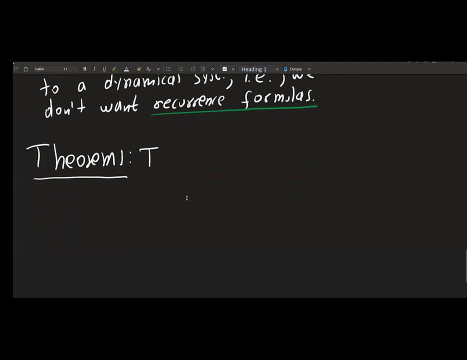 And the theorem is is: is this one? So it's basically the solution of some dynamical system, So the solution of the linear dynamical system. this is a linear dynamical system because there's no, everything is. 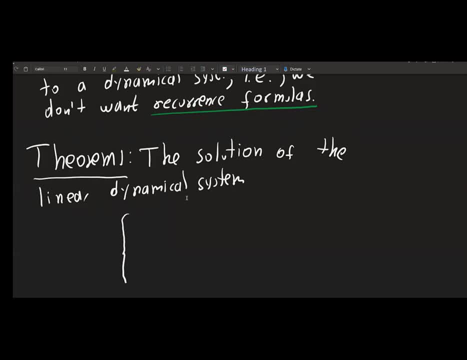 the recurrence formula is linear, So it's gonna be like this: a n plus one is equal to r, where r here is gonna be a constant times a n. So in this case, this r that is here is non-zero constant. 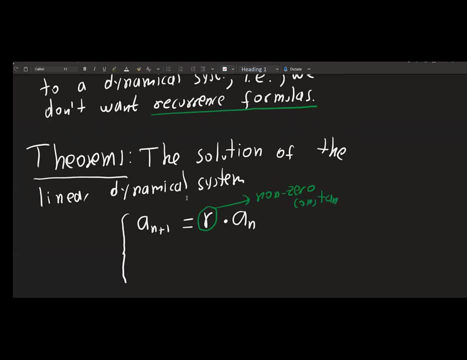 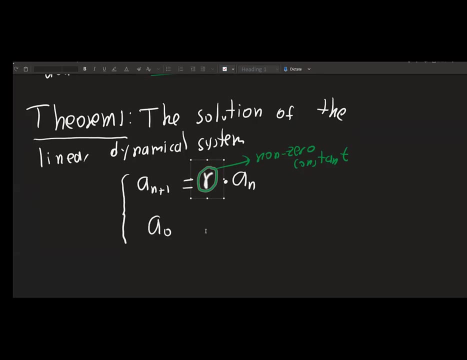 Now the reason that I'm we are asking for non-zero is because if it is zero, if this is zero, then pretty much all the terms of the sequence are gonna be zeros, And then a zero is gonna be some constant. 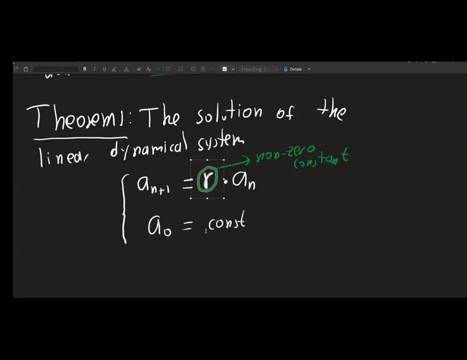 a zero is gonna be some constant. So what we have here is this is this: here is a special case of a linear recurrence formula where a n plus one is just a constant times a n. There's no other constant here. 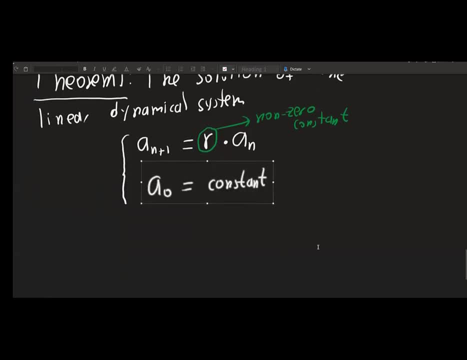 And a zero, of course, is a constant. That's the initial condition. So if that is what you have, then is the solution, which means the closed formula is gonna be this, The nth term of that sequence? 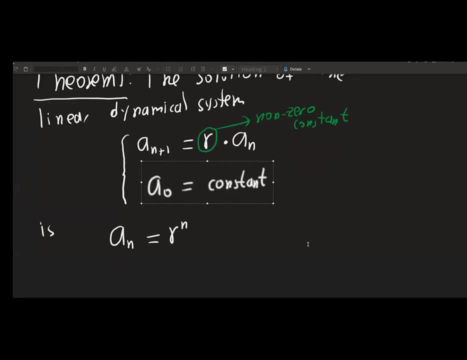 is actually equal to r to the n times the initial condition. So what that is saying is this: The sequence that you get from this dynamical system or this linear recurrence formula that we have here. that solution is exactly the same as this one. 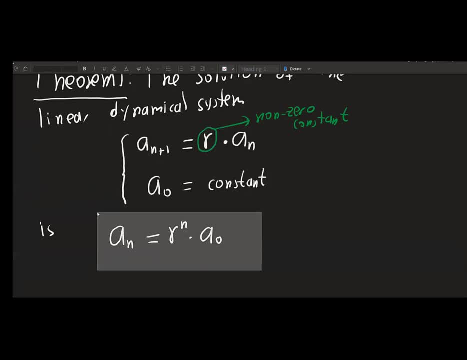 So you hear in the this one that I'm highlighting that's not a recurrence formula, That's what we call a closed formula. So it does not depend on the previous one, It only depends on r, zero and the value of n. 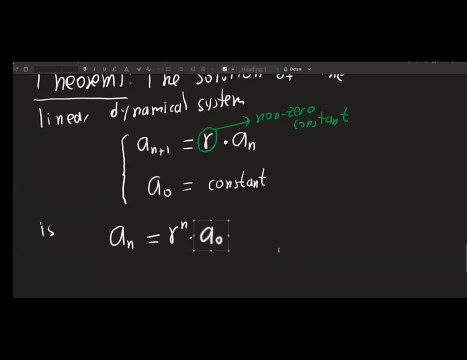 Okay, All right. So let me go back to the example we did at the beginning of the last lecture. So the example, So let me just recall that. So the example we had, So first example in the class. So if you remember that, that was from: 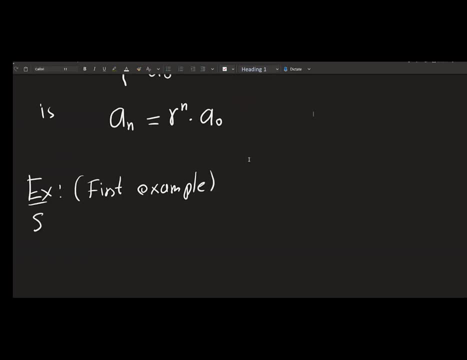 the savings certificate. So we had the, the savings certificate. This is the one that we didn't withdraw money. This is the one that we had. So the the initial initial amount was 10,000.. And the interest. 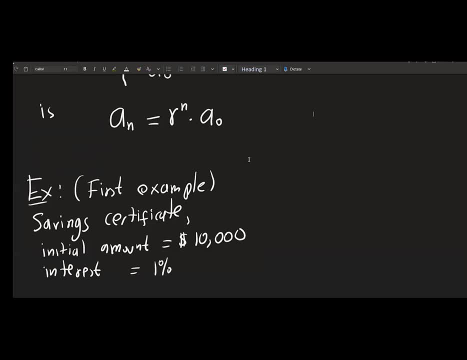 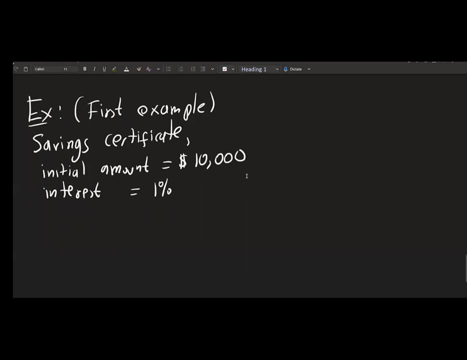 was at 1% there. So that's the one, the very first example we did in in the in the in the lecture last time, And so there were no deposits, There were no withdrawals. You just leave the money there. 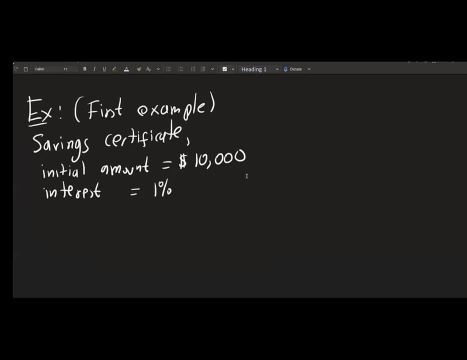 And if you remember from that example the difference equation, in that example the difference equation was this one: It was AN plus one equals to 1.01.. AN and A0. is equal to 10,000. 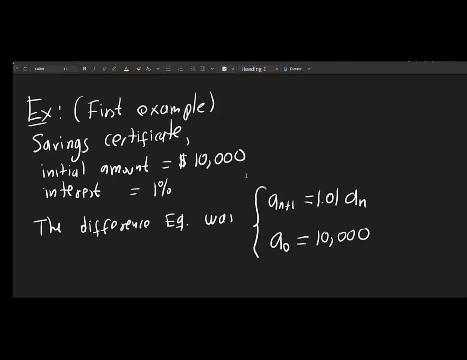 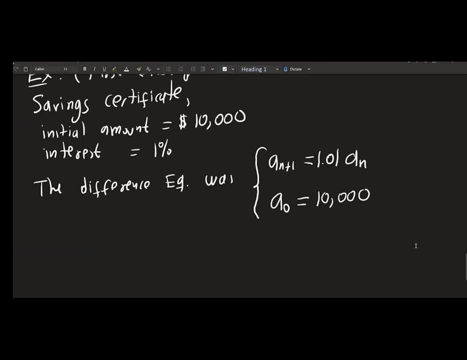 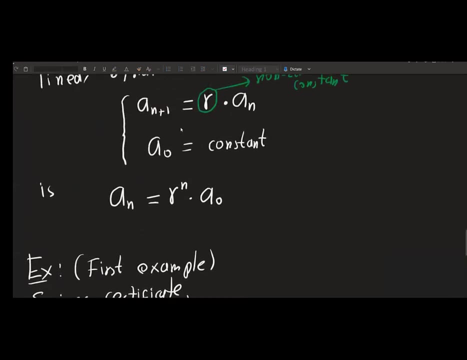 Okay, Now I I went faster here because we did this example last time- Okay, So if you look at this, this system that we have here, that's exactly the system of the theorem. So I have AN plus one. 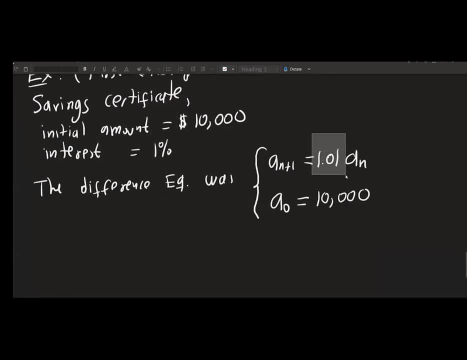 equals to a constant R and in this case the constant R is 1.01.. AN and then A0.. is just the constant, the initial value of that system, which is 10,000.. So what we can say here. 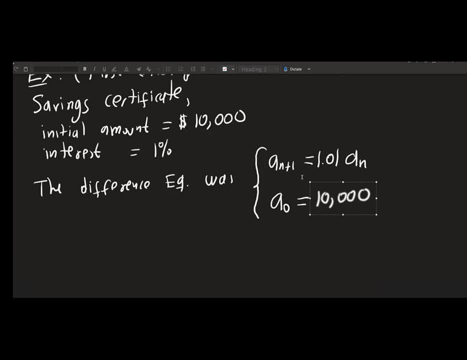 is from that theorem. so so let me just indicate this more. This one here, 1.01.. does the value of R? So so let's say this: from the theorem. so from the theorem, we know that AN. 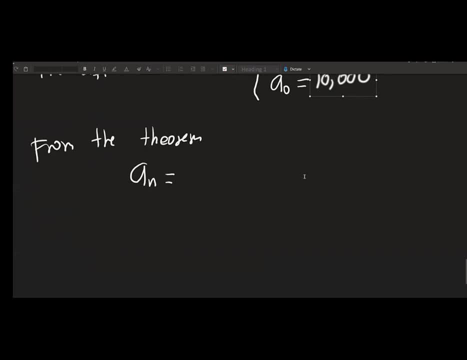 let me scroll up here a little bit. so from the theorem we know that AN is equal to R, but R in this case is 1.01.. to the N times the value of A0. which in our case, 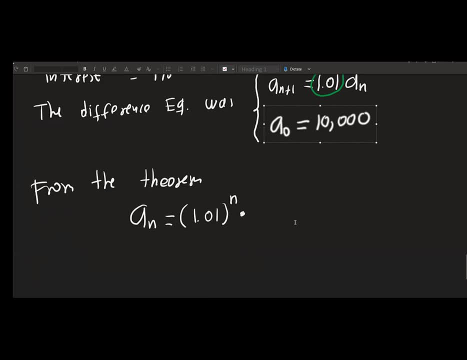 is $10,000.. So multiply it by $10,000.. Okay, Or, if you want to write it down a little bit better, I'm going to put the $10,000 up front. so $10,000.. that multiplies 1.01.. 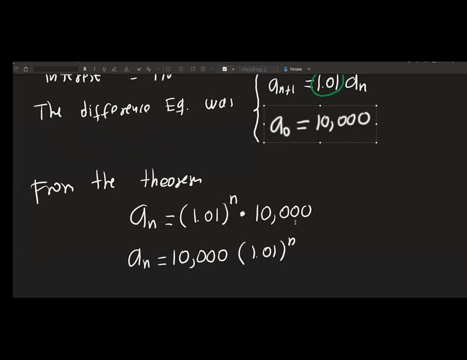 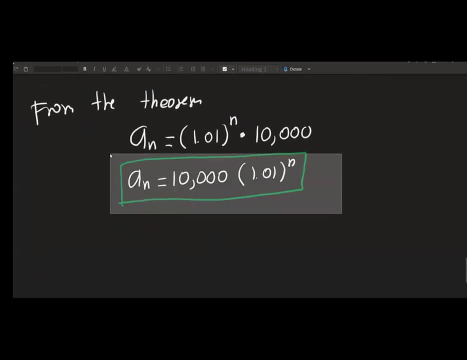 to the N, And so this is going to give us. it's exactly the same sequence. it's just that this one here right now is the closed formula. Okay Now, so let me, let me just put here: 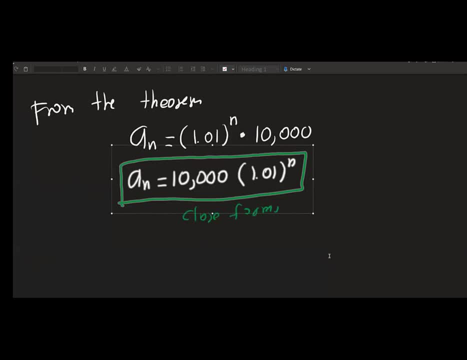 closed formula. So that's what we call the closed formula. Now, what is the advantage of this closed formula? The advantage of this closed formula is that, for example, if I want to know what is A of 100. I just have to plug in. 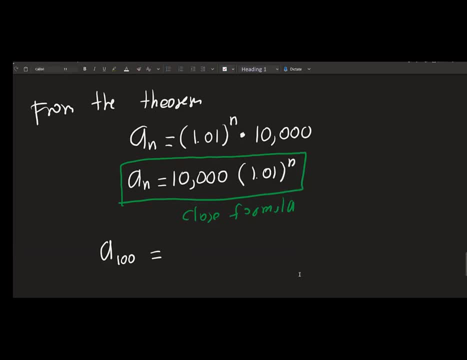 here the N for 100.. So it's going to give me $10,000.. that multiplies 1.01. to the 100.. and I just compute that and I will get, and I will get the value. 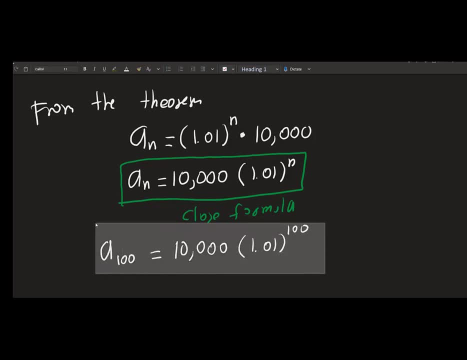 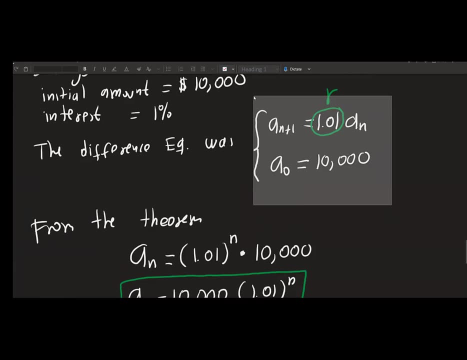 of A of 100.. Now, if you do that with the recurrence formula, just ignore all of that and just do it with this if you want the value of A100.. you need to compute the value of A99.. A98.. 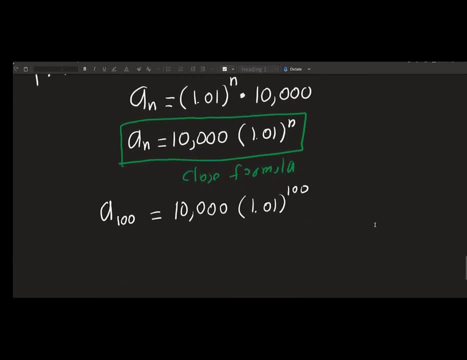 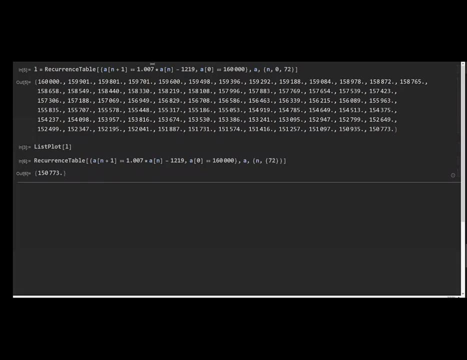 and so on. Now, if you use Mathematica, Mathematica is going to do the same thing. If you just let me come here, if you put this in Mathematica Mathematica, what it's doing is well, it's just compute. 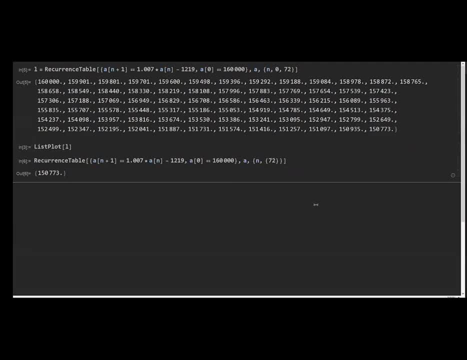 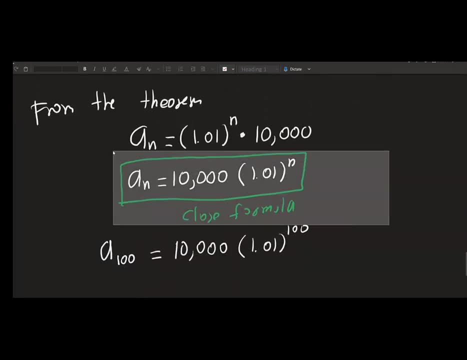 the recurrence formula and goes to all that because it does it very quickly, but it's still using the recurrence formula. The advantage of the closed formula is I don't have to know all the previous computations to be able to know. 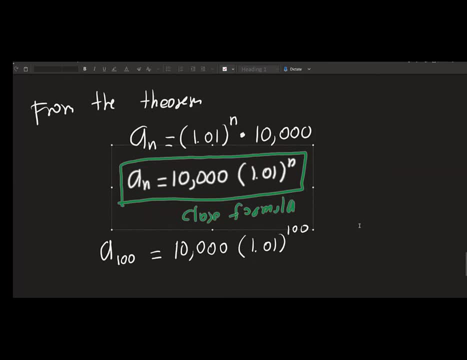 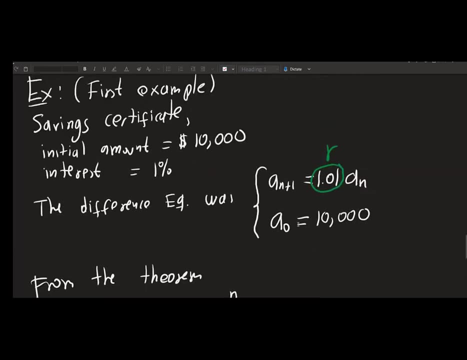 what is the value of any particular AN? Okay, All right, So we're going to move into another example, and so we're going to, whenever we can, we're going to make use of of this theorem because 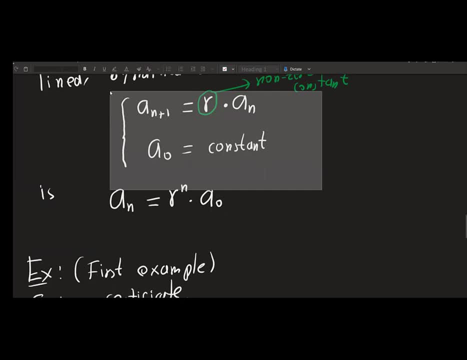 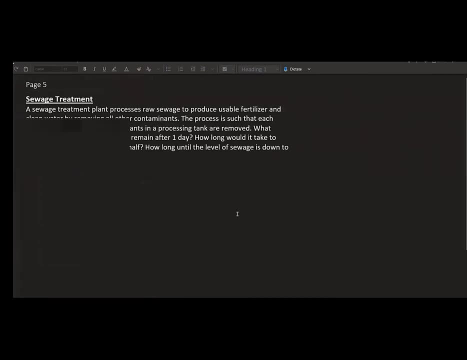 then we don't have to do this with the recurrence formula. All right, Now let me move into the next example. Okay, so so let me let me read this one. So this is the sewage treatment. So what we have here is: 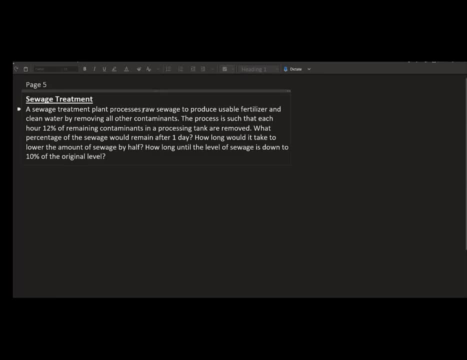 let me read So. a sewage treatment plant processes raw sewage to produce usable fertilizer and clean water by removing other contaminants. The process is such that each hour, 12% of the remaining contaminants in a processing tank are removed. 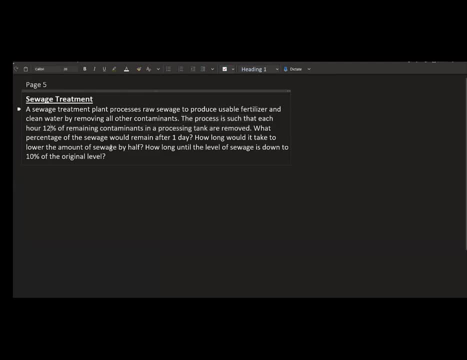 So every hour, 12% of the contaminant is being removed from that plant. So there are several questions here. The first one is this: What percentage of the sewage will remain after one day? So we need to answer that question. 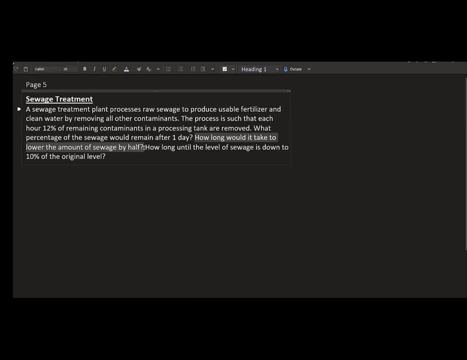 Second question is: how long will it take to lower the amount of sewage by half, So the contaminant by half? That will be the second question And the third question will be how long until the level of sewage is down? 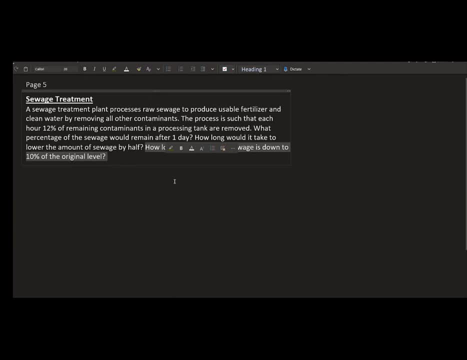 to 10% of the original level. So let's look at the solution then. So before I go into the solution, I want to point out something here in the statement- And there's nowhere in this statement- they are telling us: 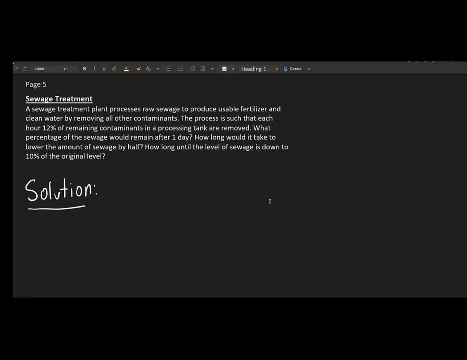 what is the initial amount, Or A0. in this case, So, when that is not given, just treat A0 as a constant. So A0 for us here will be the initial amount. so this will be the initial. 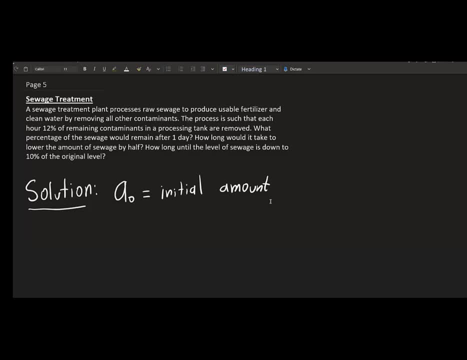 amount of the contaminant in the tank. So that will be A0.. We don't know what that is, but that will certainly be a constant, And so let's give a name for AN. What is AN, So AN will be the. 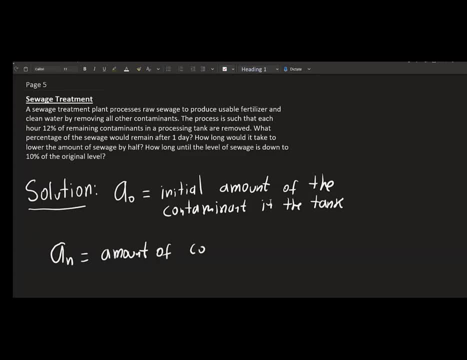 amount of contaminant in the tank after after N hours. So that will be the contaminant after N hours. Now, whenever you are doing this problems, always choose correctly what your AN should be, Because that's going to make a difference. 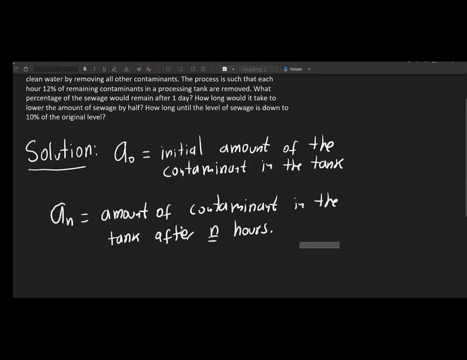 when you are trying to solve these problems, Choosing AN correctly, what the correct meaning for AN is important here. Alright, so let me try to to draw a picture first, Before we actually go into setting up the recurrence formula. 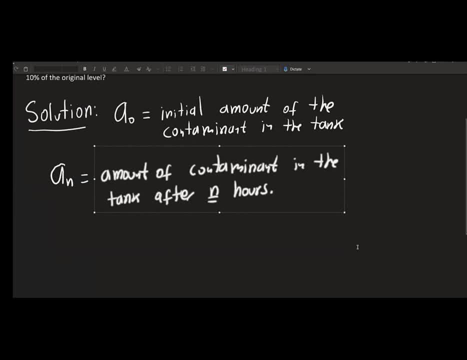 of the problem. So let me draw a picture here. So you're going to start here at A0. Which we don't know what it is, And in the first hour, So according to the problem, the contaminant is going to reduce. 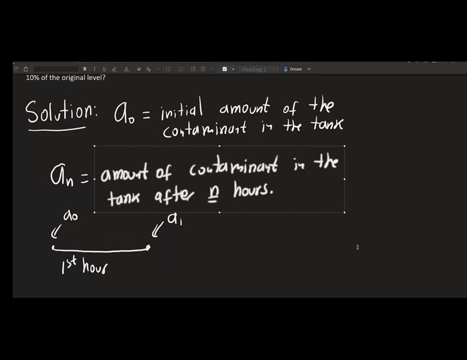 and it's going to reduce up to the A1.. That will be in the first hour, So when you are here, in the general case, this is the AN And this is going to be the AN plus one. So this will be the general case. 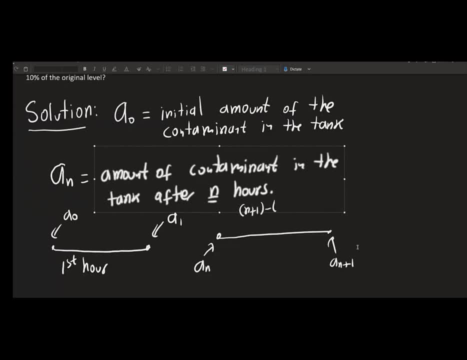 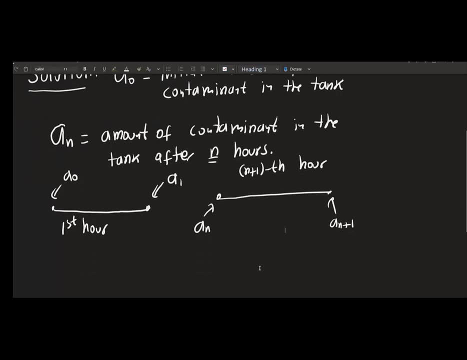 This will be the N plus one hour. That will be just the picture that we have here. So this is the initial amount of contaminant after the first hour will be A1.. And this is on the during the N plus one hour. 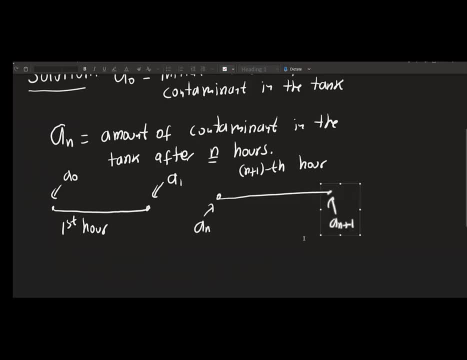 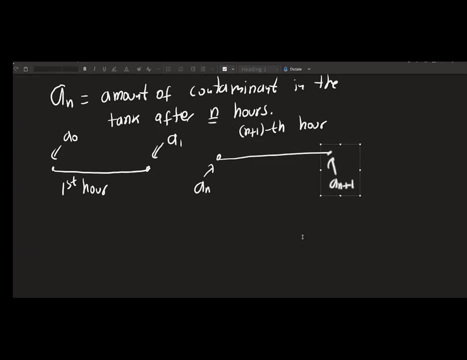 initial amount of contaminant is AN, And it's going to end up in AN plus one, Alright, So let's look at the equation here. I'm going to write down this in English. So: contaminant, The contaminant. 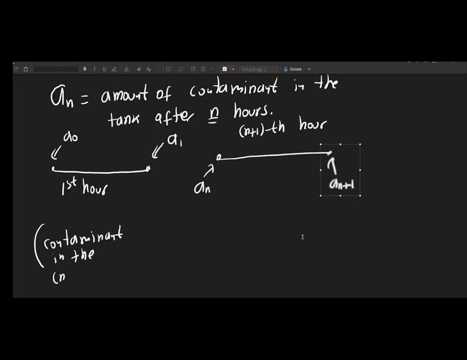 in the N plus one hour is going to be equal, Because I want to set up this as an AN- Which I remember is the future Here- As a recurrence formula. Let me go back and read. Let's read the problem again. 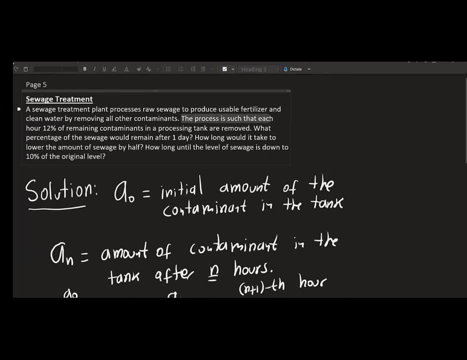 So what is happening in the problem here? So let me read this sentence here: So the process is such that each hour, 12% of the remaining of the contaminants in the processing tank are removed. So every hour, whatever is left of the contaminant. 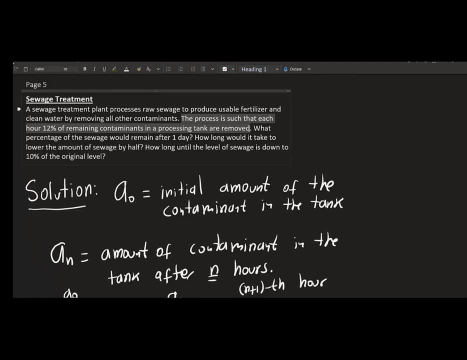 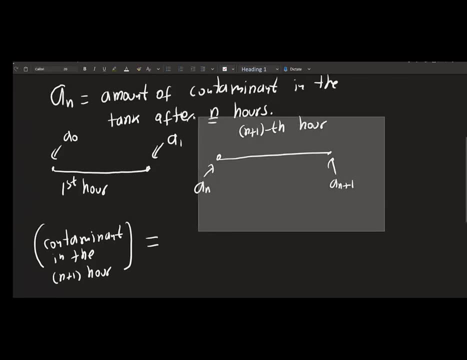 at the beginning of that hour, 12% is being taken away by that tank. So the contaminant in the N plus one hour, which is this part, will be equal to whatever the contaminant we started with, minus 12%. 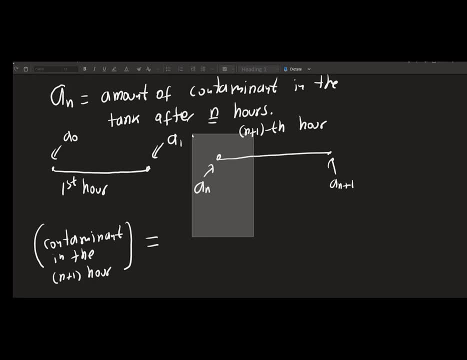 of this one, Of this one again, Because we are taking out 12% of whatever we started with in that hour, So this is going to be the contaminant. And because we are looking at this, at this, AN right here. 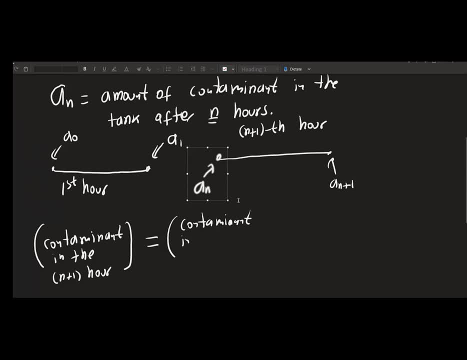 is the contaminant in the nth hour. in the nth hour minus, then we are reducing in this hour 12% of, of course, the initial contaminant, which is this one here. So that's going to be minus. 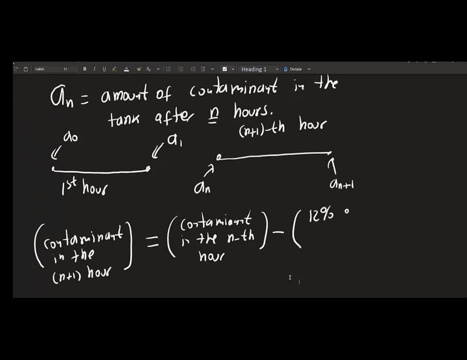 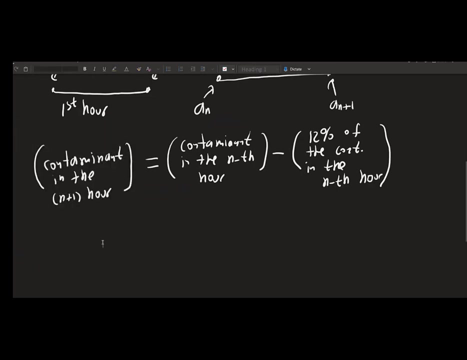 12%. the contaminant in the nth hour. Alright, Alright. so what is this one right here? This is AN plus one. The contaminant at the end of that hour. So then, this is going to be AN plus one. 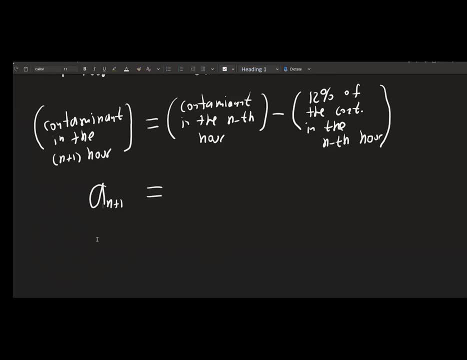 Let's give it a second there to update, And that's equal to the contaminant at the end of that nth hour, which is AN. So it's going to be AN Minus And that's going to be minus. 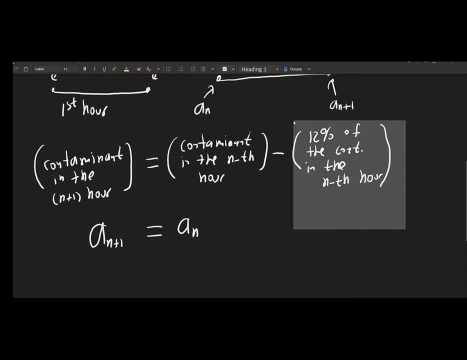 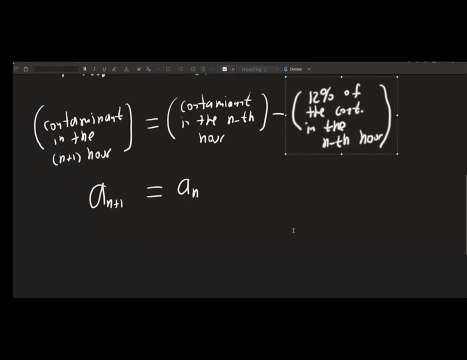 this one here, this 12% of the contaminant there at the end of that hour. So it's going to be minus 12% of that. So that would be 12% of AN, which is going to be. 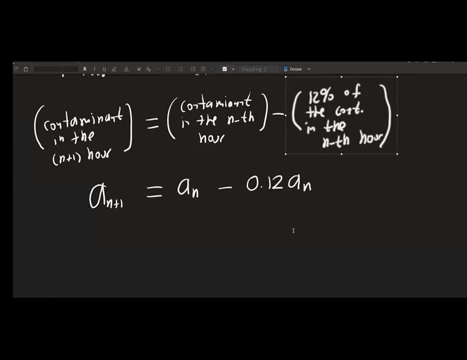 0.12. AN. So let's simplify things out here. So the AN plus one is going to be equal, So just do this abstraction here. So one minus .12. is equal to 0.88.. 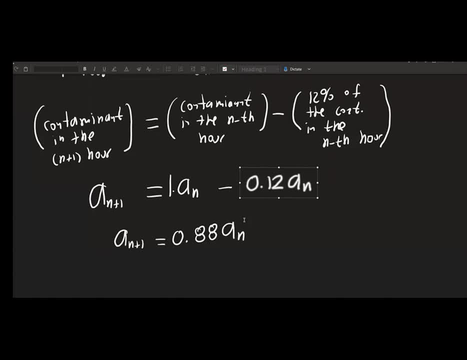 of AN Right And so, And so we will have the dynamical system or the difference equation. if we knew what A0 is. but A0 is just a constant here. Now you're going to see that we will need. 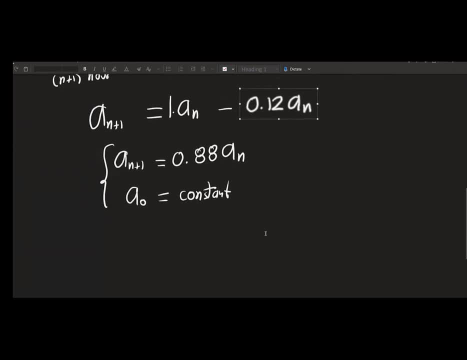 that value of A0 to answer the questions we are trying to answer. So that would be our dynamical system or difference equation. Okay, now here, because we already have a theorem that tells us what this is. 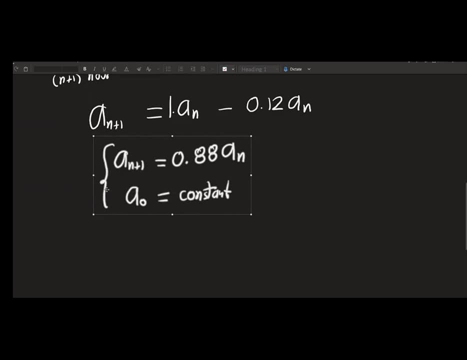 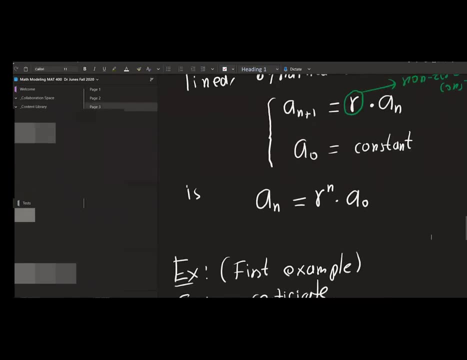 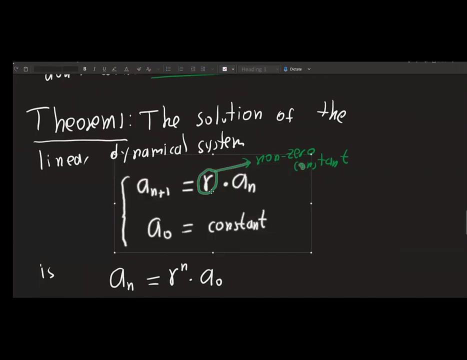 Now, this one here is exactly the theorem we had at the beginning of the class. Let me go back here to to this one. So right here we have AN plus one equals to a constant, which in this case is: 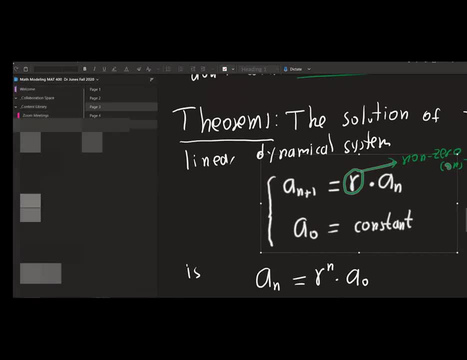 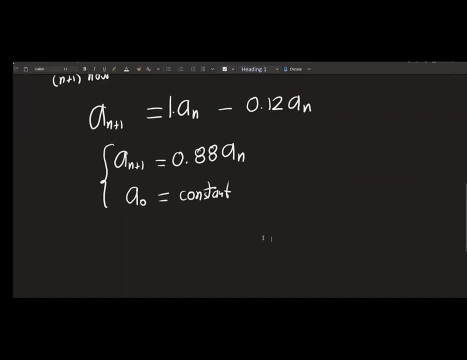 in our case is 0.88.. and A0 is a constant. So if I go back here I have that theorem In this case, then this constant that is here, 0.88, is our R. So let's write down: 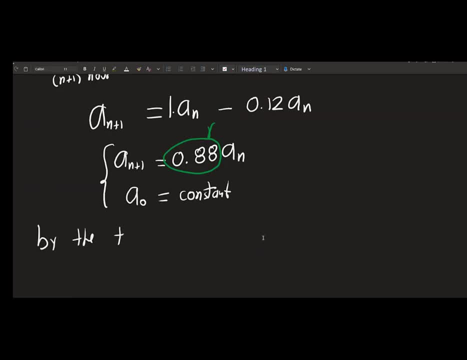 by the theorem. What is then AN, Our closed formula for this, for this example? So that's the closed formula. Alright, So what do we need to answer here? So now we have the closed formula. so that means it's going to be a little bit. 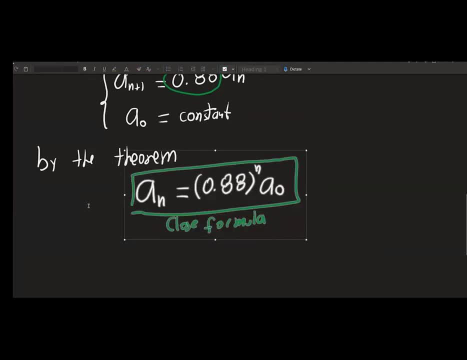 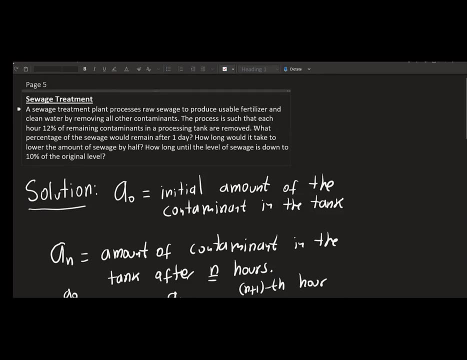 easier to solve things. It's not a recurrence formula. Let me scroll all the way up here to go back and see what questions we have. So our first question is this one: So what percentage of the sewage will remain after one day? 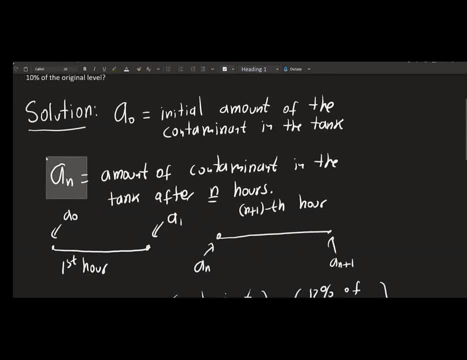 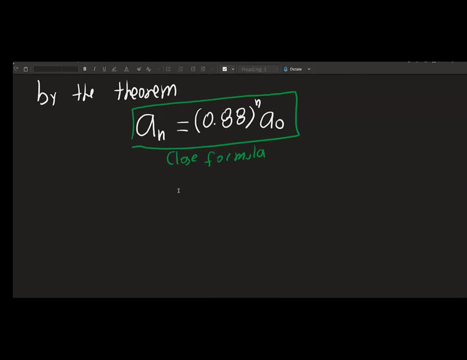 Now remember the this AN that is here is measured in hours. So what we really want here is we need A of of 24.. So A of 24.. we just basically just plug it right here. No need for. 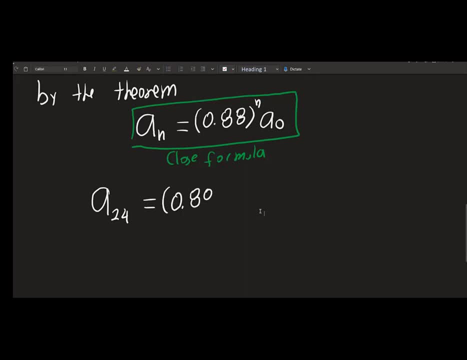 recurrence formulas, It's going to be 0.88.. to the 24. times A0.. And so, in this case, well, you probably have to use the calculator for that, or Mathematica, And this is going to give you. 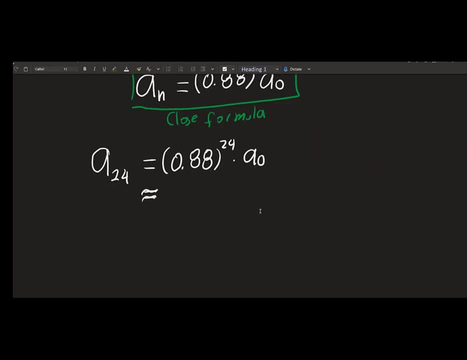 approximately 0.05.. 0.05. of A0.. Now let's make an interpretation of what this actually means. So after 24 hours we have 0.0. of the initial amount. So 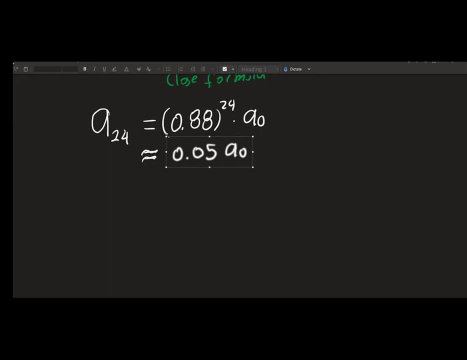 what is remaining of that contaminant after 24 hours? In terms of the percentage, After 24 hours, only 5% of the initial contaminant remains. Okay, so that will answer the first. 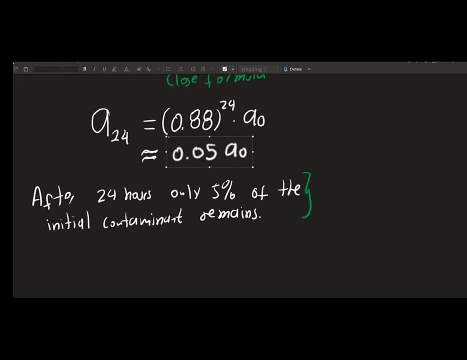 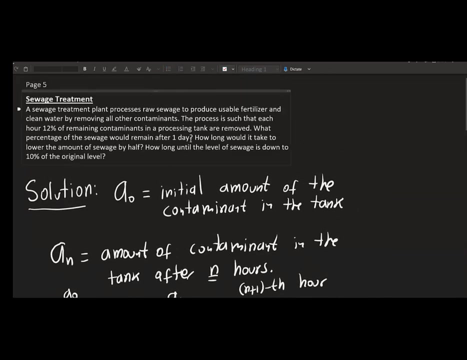 question. So this here was question one. So this was question one, Okay, Okay, Let's go to the second question. The second question is: how long will it take to lower the amount of so just by half? 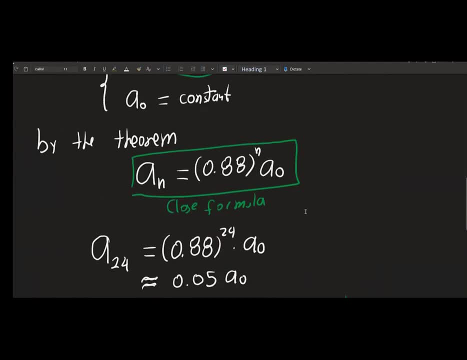 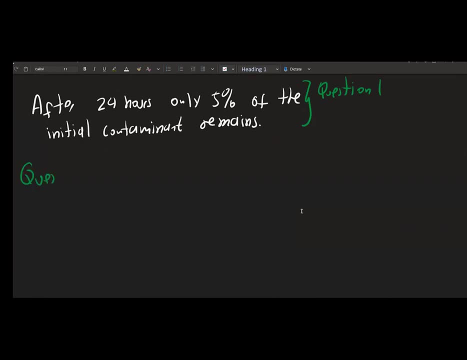 So they're asking me here for time. So for the second question, let me put this down here. So for the second question, this will be question two. Question two: This is asking for time, Time Now. So what we're doing is: 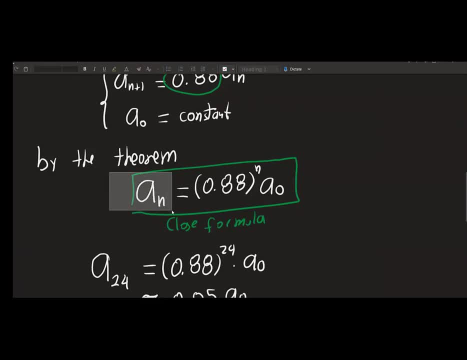 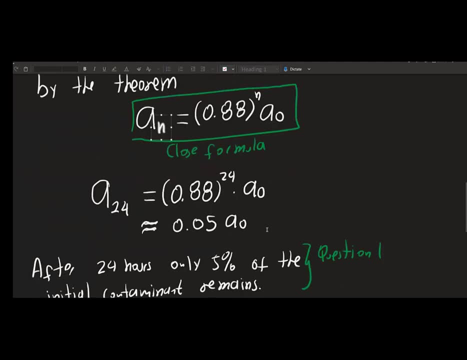 we want to have n, Right, We don't want a n, because that's the amount of contaminant left. What we want is n Here The time. So we want time, Which, in this case, we are measuring. 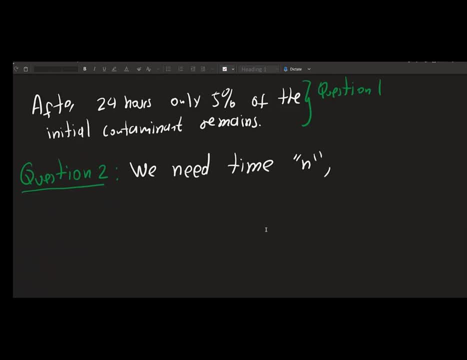 by n. So we need to find. So we need to find n, Because in this case n represents time Such that, such that a n as a fraction here. So it's going to be one half of a zero. 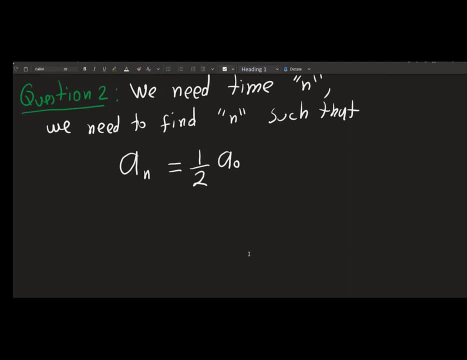 Now, this is an equation that we need to solve for n. Okay, Now, n here cannot be in terms of a zero. We are looking for a specific time. So, even though we don't know a zero, because we have, 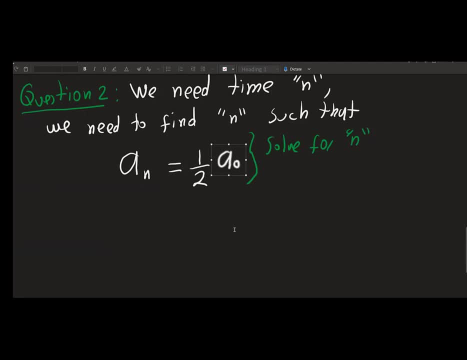 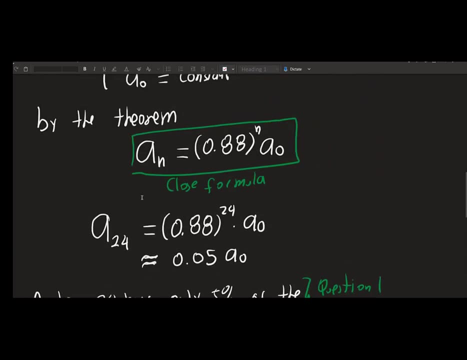 a closed formula, we'll be able to solve this exactly. Now let's go back to a closed formula for a n. Let me scroll up here: This is the formula for a n, So a n here can be replaced. 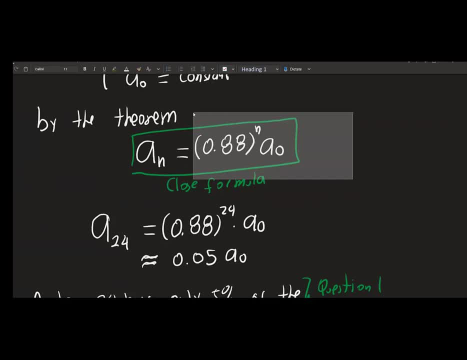 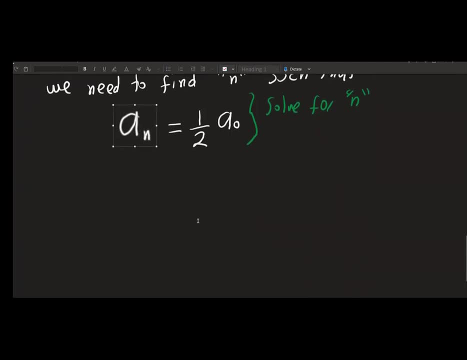 by this right hand side, And that's exactly what we're going to do for this part. So we're going to do that here. So that's going to give us a 0.88.. to the n: a zero. 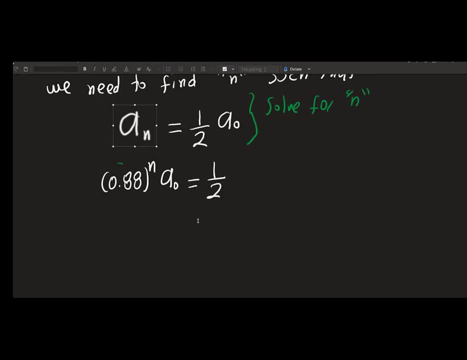 equals to one half of a zero. Okay, Any questions about that? Any questions? Remember, we are looking for n here, Right? We are looking for n. Okay, so this is the part where I'm going to ask you. 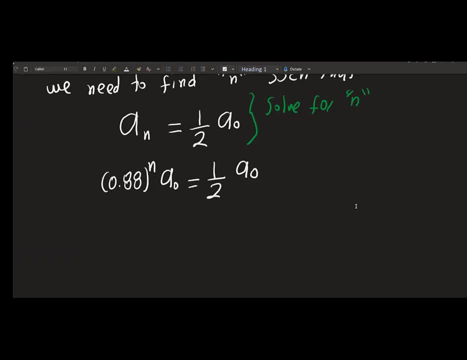 to work on your own a little bit, So I'm going to give you a couple of minutes. Please work on solving this equation for n. So do it on your own And I will check with you a couple of minutes later. 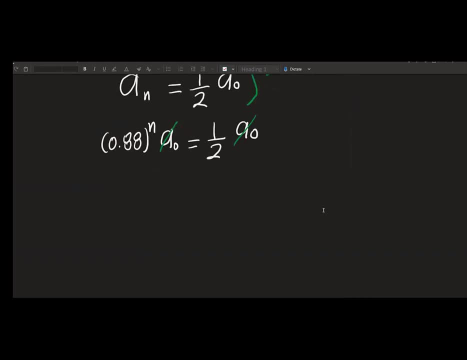 Okay, So work on solving this for n. So this is the log of that to the n equal to ln of 0.5.. And then this n that is here comes down as a multiplication, So it's n? ln of. 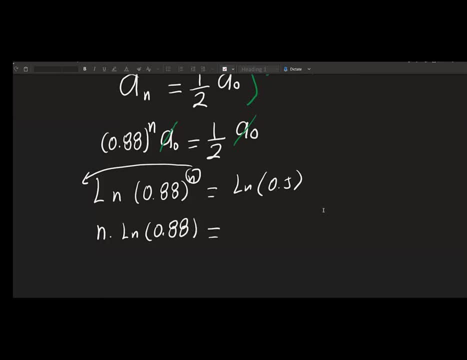 0.88.. equals to ln of 0.5.. So n here would be equal to ln of 0.5.. and this is all divided by ln of 0.88.. It's that number here. 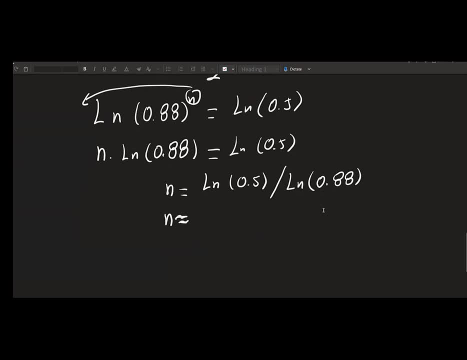 So an approximation of this- Okay, so now we get this- is 5.42. So let's answer the question. So it takes 5.42. hours to lower the contaminant by half of the original. 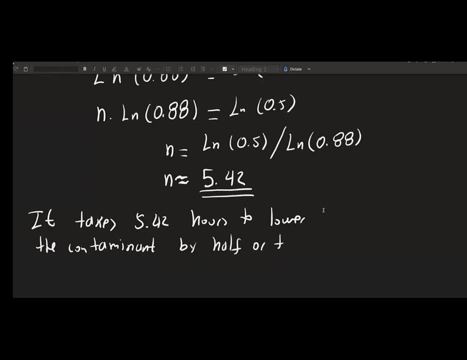 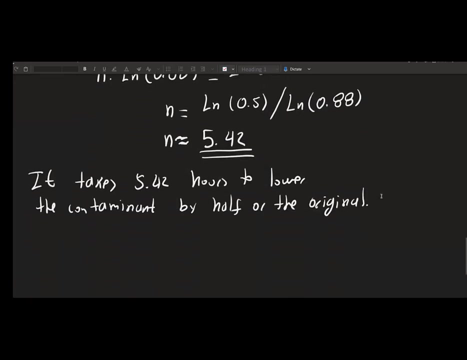 Now you see, in this, in this example, we didn't need a 0. Because anyway a 0 is going to cancel here anyways. So that's why we could solve the problem. Also. one more thing I want to mention here. 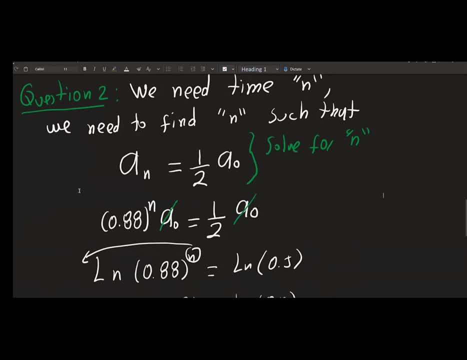 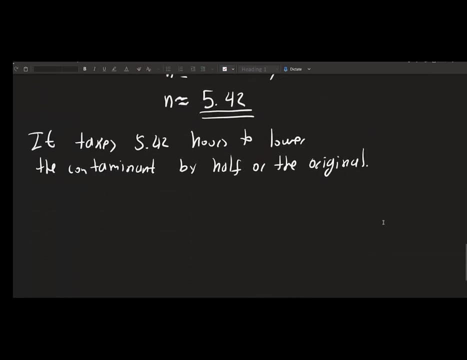 If we didn't have the closed formula for an, then this problem would be a lot more difficult. Okay, so having the closed formula gives us an easier way to solve this problem. Alright, let's look at the third. 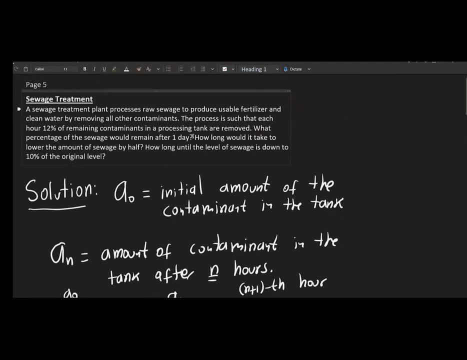 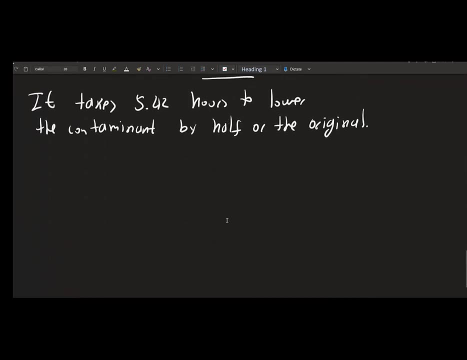 question. So the third question is: How long would it take to- Oh, this is the second one- How long until the level of sewage is down to 10% of the original level? This is actually very similar to question number 2.. 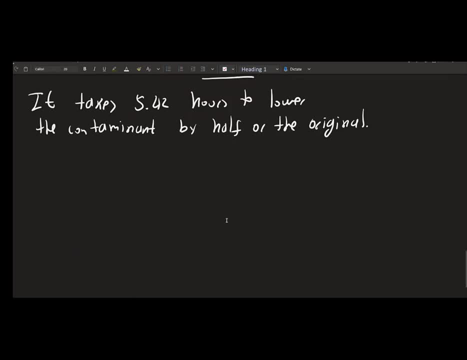 Let's see why. So this is going to be question 3.. So, question 3.. So we still need to find time here. So we need to find time, Find time And in this case, for us, time is. 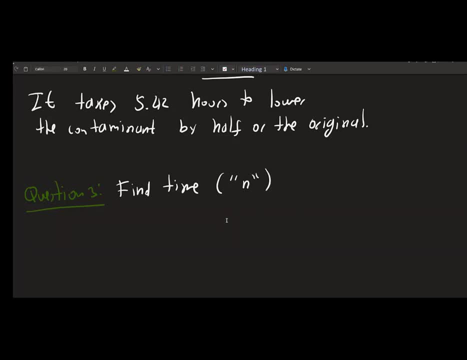 our variable n. So we need to know what is the time. so that is 10% left of the contaminant. So what would be the equation here? a n, Alright, so we're going to do. 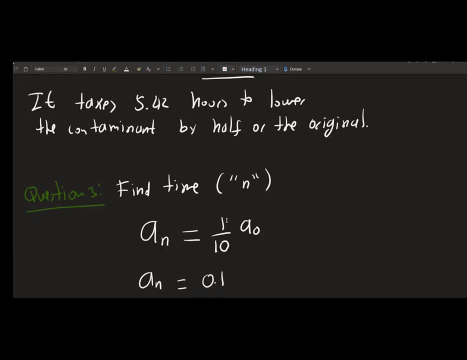 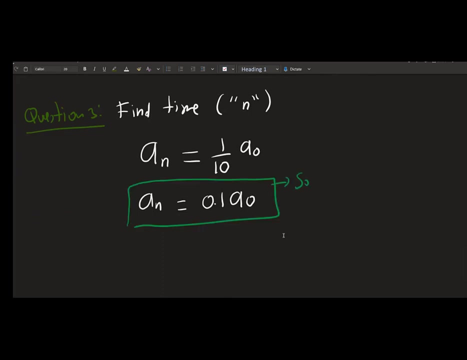 something similar here. Alright, so this is similar to what we did the other one. Again, I'm going to give you a couple of minutes and please solve this for n, And then we'll compare the answers Solve for. 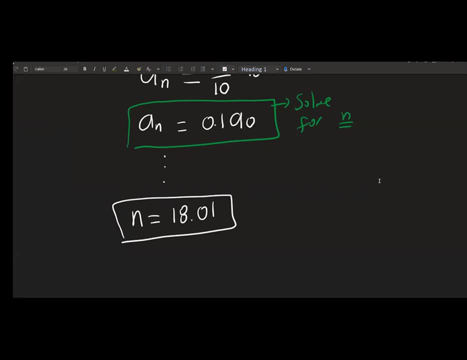 for n, So that is hours. So let's answer the question. So it takes. It takes 18.01 hours. Okay, guys, I'll see you then next week.